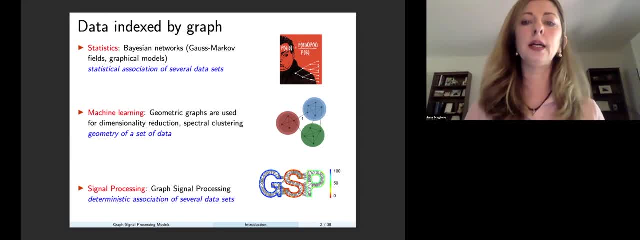 In machine learning, it is also very common for high dimensional data to seek a lower dimensional structure, emulating it through geometric graphs. Graph signal processing is a relatively newcomer in this field And the idea is essentially to provide a deterministic association between several data sets. that generalizes digital signal processing, both time series analysis and multidimensional image analysis. 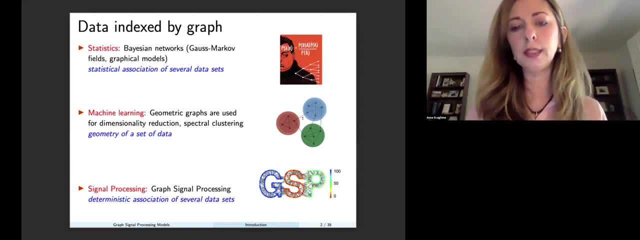 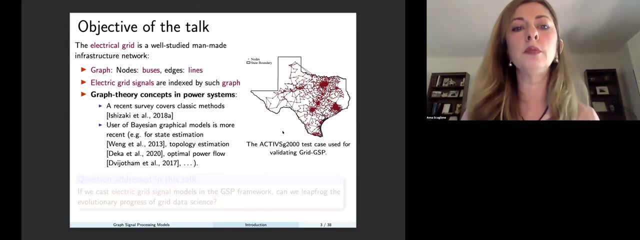 by essentially generalizing these concepts to data that lie on an irregular support such as a graph. So the electrical grid, obviously the physical system is well studied, based on the laws of physics. In this case, the nodes are the basis of the system and the edges are the line of the system, and electric grid signals, essentially, are indexed by such graph and focus on signals that are indexed by the basis, in particular the state of the grid. 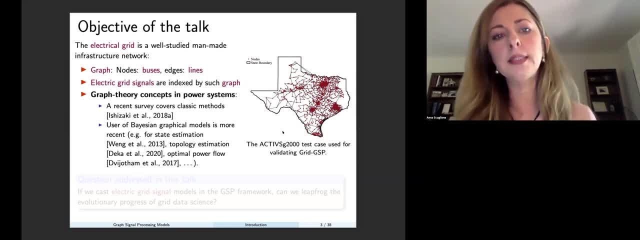 And graph theory concepts are an integral part of the analysis because they are essentially in the fundamental equation that express the relationship between these electrical quantities. There is a recent survey in 2018 that covers sort of classic methods of dynamic power system analysis and they are clearly well connected to graph theoretic concepts. 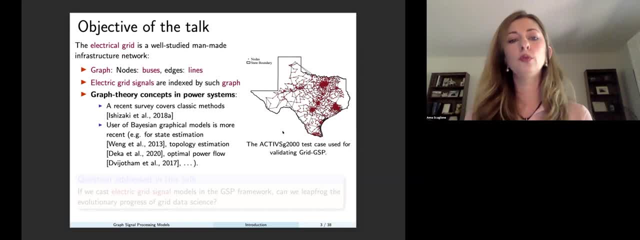 But more recently people have tried to apply toolboxes from machine learning and, in particular, Bayesian graphical models for a number of different problem formulations and applications. GSP, instead, is something quite new And it's something that I've been paying attention to because of my interest in the GSP framework in general. 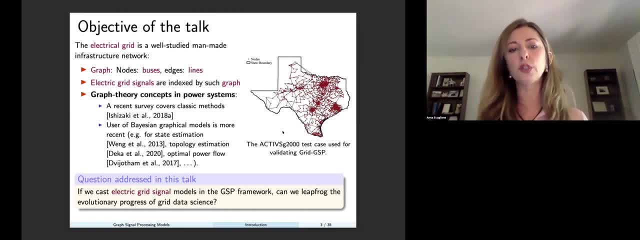 And so the questions I'm trying to answer in this talk is: obviously, I'm not going to change the laws of physics that describe the electrical signal, but what I'm going to do is to cast electric signals in the GSP framework, And the question that I want to address is: can we leapfrog the evolutionary processing grid, data science? because we can use a lot of tools that are developed in this GSP framework. 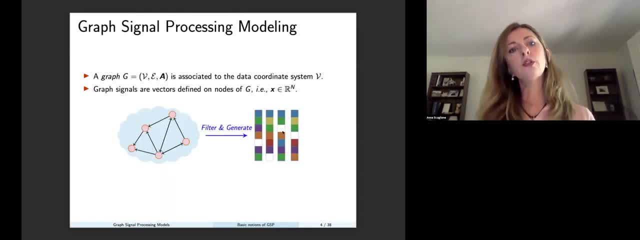 GSP data science framework in general. So what is the difference? What do we mean by data that have any regular support? A graph, in this case, is associated to a set of data points that have coordinates that are going to be the nodes of the graph, And this graph is also described by, obviously, a set of edges and a weighted adjacency matrix. So, if we have several observations, 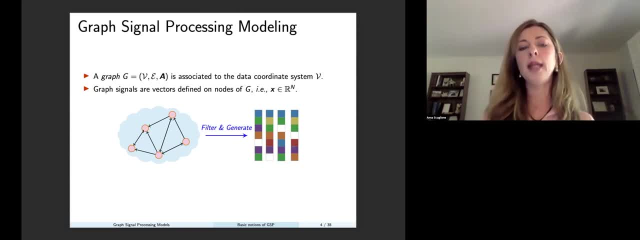 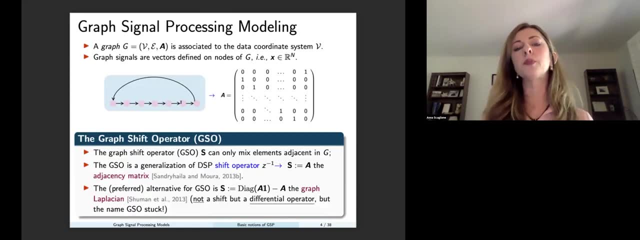 it will be these vectors And basically the way the data are generated is tied to this underlying structure, And the idea stems from thinking about the particular graph that can justify all the algorithms, and particularly Fourier analysis, for digital signal processing. As you can see, here is a circular graph. Most of the GSP is based on the idea that you analyze finite sequences and 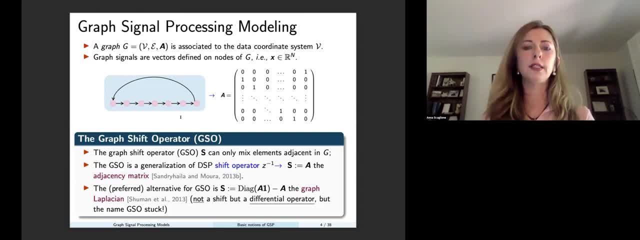 the DFT is in fact considering these finite sequences, extending them to periodic sequences. In this case, the adjacency matrix is a simple shift, And the whole idea of generalizing Fourier analysis and filtering methods to graph signals relies on the definition of what is called the graph shift operator. I will denote it with the matrix S And S can only mix elements of the graph. 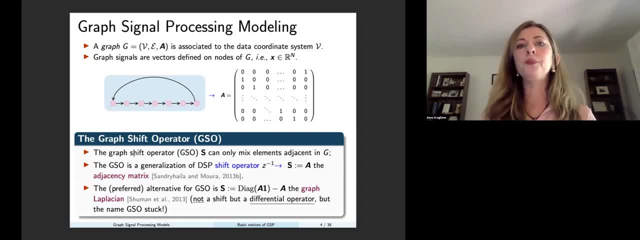 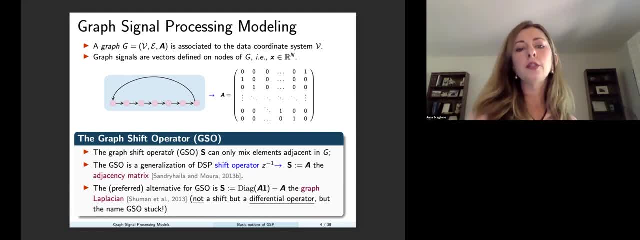 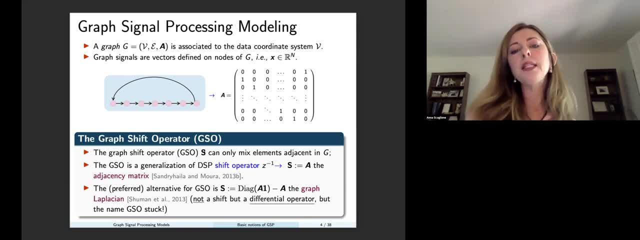 are adjacent in the underlying graph And it's basically the generalization of the shift operator Z to the minus one, In this case S would be effectively these adjacency matrix And, as you can see here in the circular graph, the shift is a directed graph, The preferred alternative. 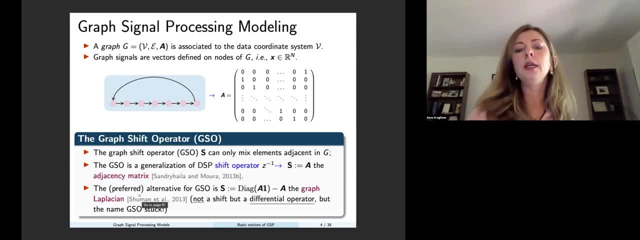 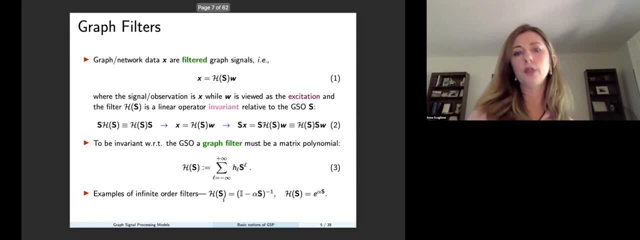 though these days is in fact a graph Laplacian, which is not a shift but is a differential operator. Nonetheless, the name GSO stuck, So I will refer to it as a GSO. The idea of a graph is that there is an input output relationship, which I express in equation one. as an input, 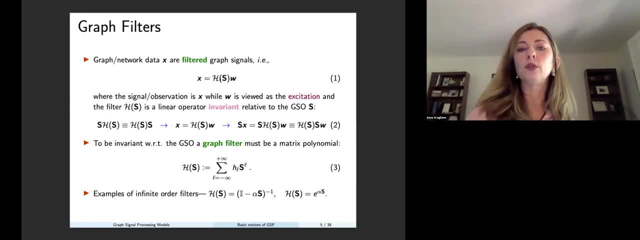 excitation W And this matrix operator H, which is a function of this GSO that describes the data essentially, And the particular property that is desired for graph filter is that they are shift invariant, just like linear time invariant filter in DSP, In other words that 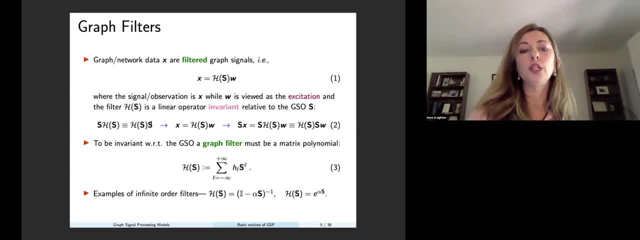 if you pre-multiply H times the GSO, you get the same result as post-multiplying it by the GSO, And that means essentially that if you shift the input, just multiply it by the GSO, you obtain the shifted output, which is true, as I said, for linear time invariant. 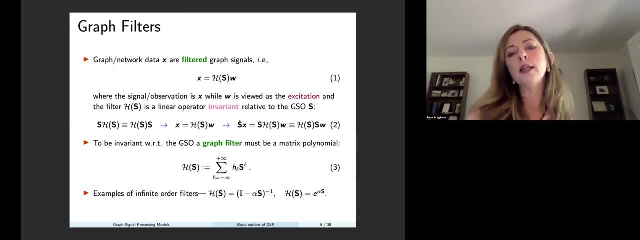 filters. So this condition actually implies that not all operators are graph filters, but only matrix polynomials, where the matrix is the GSO, And these matrix polynomial can be also of infinite order. These are two examples of infinite order filters, In this case S. 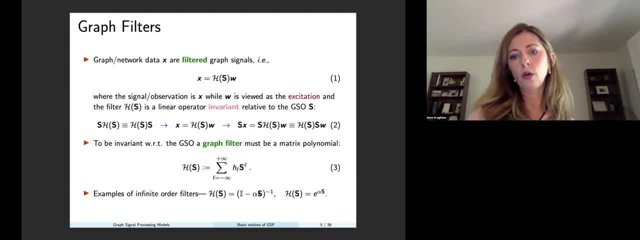 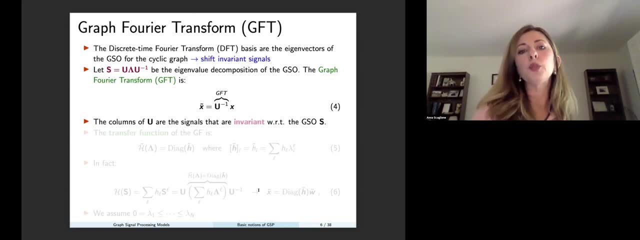 the matrix S is assumed to have eigenvalues that are all less than one. So what is the graph Fourier transform? The graph Fourier transform is obtained by taking the eigenvector decomposition of the GSO, And the graph Fourier transform basis is nothing but the set of. 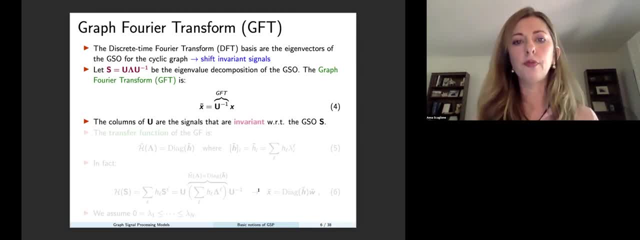 eigenvectors of the GSO itself, And in particular x tilde here is obtained by taking the inverse of the eigenvector matrix and multiplying it by s, And in particular in DSP. for the case that I showed before of the circular graph, the adjacency matrix that I've showed you, which is a GSO- 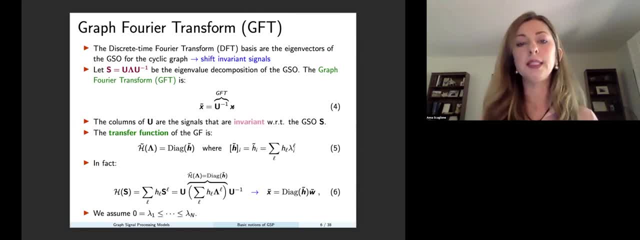 would produce exactly the DFT basis. So you can see the strong connection with Fourier analysis in DSP. Not only that, but what we find is that we can express an input-upload relationship of a graph to the GSO. And we can express an input-upload relationship of a graph to the GSO. 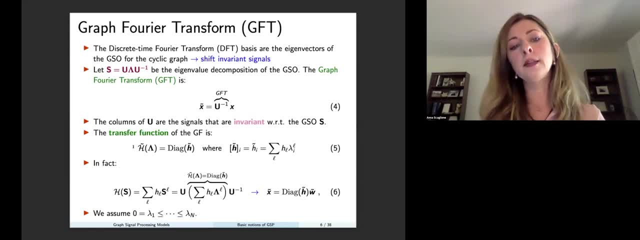 And we can express an input-upload relationship of a graph to the GSO And we can express an input-upload filter in the Fourier domain, in the graph Fourier domain, And what we obtain is obviously, since H is a matrix H of S is a matrix polynomial, that the input-upload relationship in the Fourier 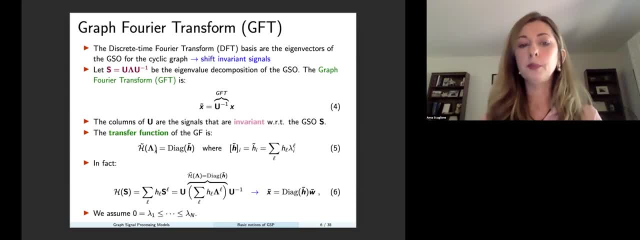 domain is going to be a multiplication, entry by entry, with what we call the graph filter transfer function, H tilde, whose elements are essentially polynomial, computed with the same weights HL of the graph filter times, each of the eigenvectors And we can express an input-upload. 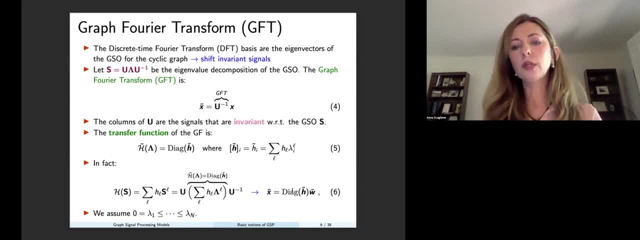 value to the power L, And so you can find here the relationship. that is also true for DSP, where in the DFT domain, the input-upload relationship is a multiplication by the Fourier transform of the impulse response. Now, since we are using the graph Laplacian, we know that. 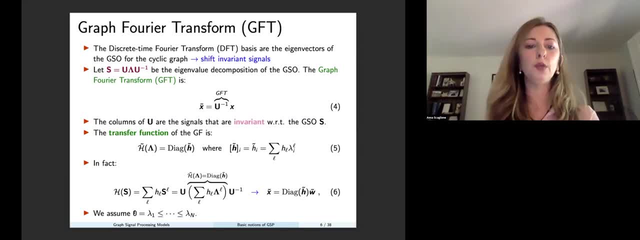 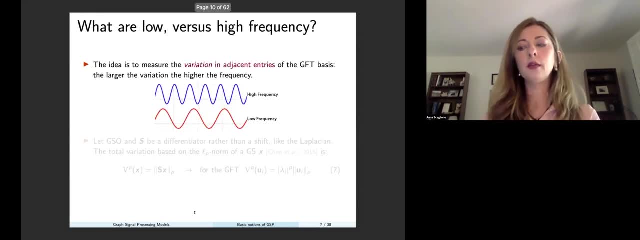 one of the eigenvectors is a constant vector. It corresponds to the eigenvalue equal to zero. So we know that the eigenvalues are ordered in increasing order. This convention is not really arbitrary. It's because it's tied to the idea of frequency and particular variation of the signal. 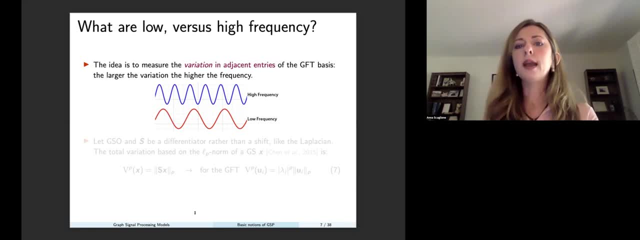 over this irregular support. So what is a high frequency or a low frequency? As we said, S is a differential operator, So we can express the notion of variation of the signal, which will be S times X. This is the norm P And in general this norm is usually the norm 2, but could be also in some cases. 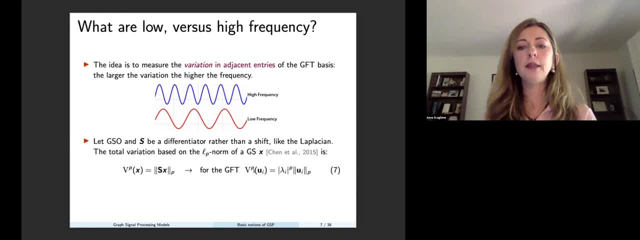 norm 1.. And because of that, if we look at the basis vector UI for the GFT, we can clearly see that, since when we multiply by S we obtain the same vector multiplied by the eigenvalue, we can see that low eigenvalues correspond to low variation and high eigenvalues correspond to high variation. 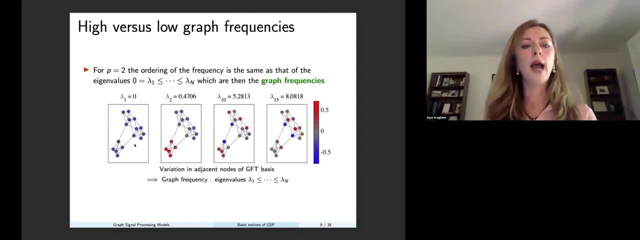 This is illustrated in this figure where we have this particular graph. Obviously, for lambda, 1 equals 0,, as I said, we have the constant vector, so it's smooth over this support. But if you progressively look at the higher eigenvalues, you can see that they tend to be smooth over different. 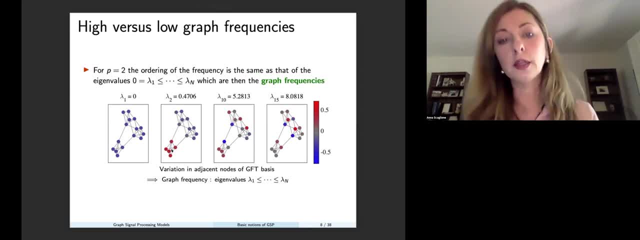 clusters of the graph And, in fact, the fact that they are smooth in different clusters of the graph is tied to a really interesting result from spectral graph theory And, in particular, the so-called result of spectral clustering, that utilizes the smallest eigenvalues to identify different communities in the graph. 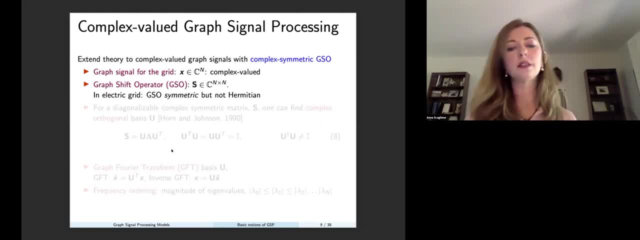 Now the grid signals are expressed as phasors, And so we are not going to deal with a real signal, but a complex-valued signal. And in particular, we see the graph shift operator is not hermitian but is actually very. 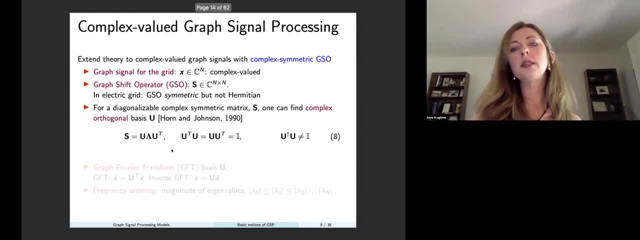 actually symmetric. So in this case we can still for a diagonalizable GSO we can find a complex orthogonal basis such that S is equal again to the matrix factorization based shown in 8, and U are orthogonal matrices And in particular the Graf-Fourier transform. 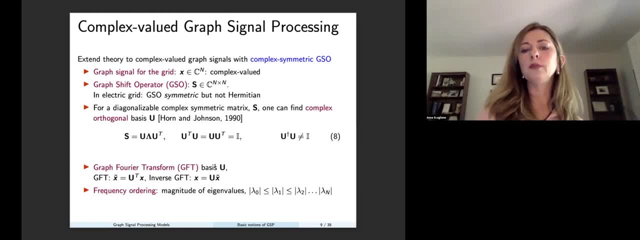 can be shown to be this basis. Essentially, this is an appropriate definition And for the graph frequencies, an appropriate definition is to take the absolute values of the eigenvalues of this particular matrix. In general, there could be dyes in this case which complicate. 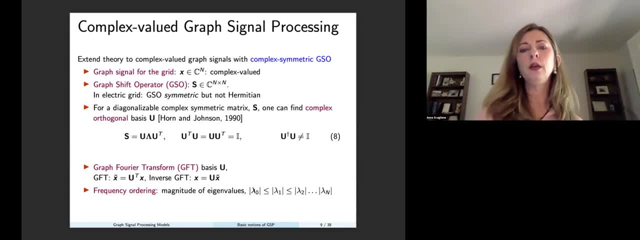 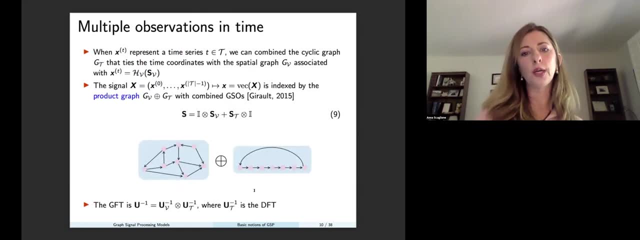 the definition, because you will have two repeated frequencies. But for the case at hand, this is just a grid case. This is really not occurring with high probability. Now, in the grid, we obviously have dynamics, So we not only have a signal, that is an option. 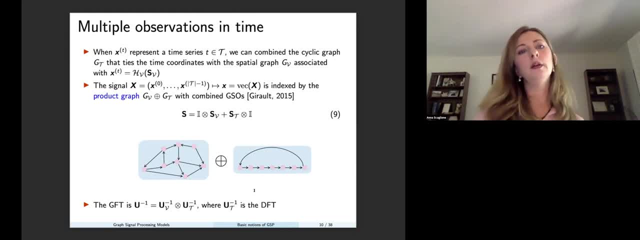 of the signal over all buses, but we also have the signal evolving in time, the state evolving in time. So let's say that we want to represent this integrated signal processing framework. As I said, time series can leverage the tools of DSP and GSP. 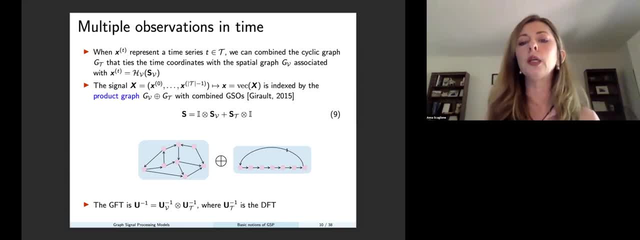 GST- sorry, indirectly- are leveraging it already because of the circular graph that describes them. So you can actually have a composite description by just essentially looking at the product graph and looking at the GSO, which is in this case, defined as a function of the GSO, of the graph that justifies the structuring space of the data and the 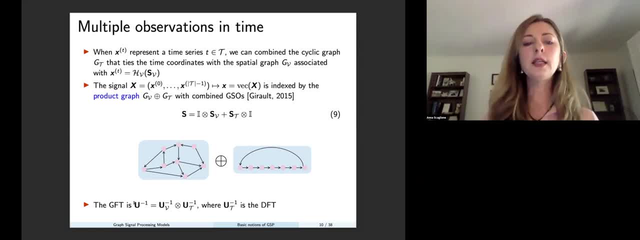 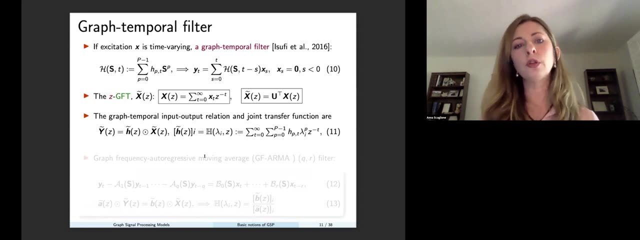 temporal graph, which is simply the Scythian's graph, And in this case, the GFT is the Kronegger product of the two bases, So the respective GSO. Now, what is a graph? temporal filter is the composition, obviously, of the two concepts. 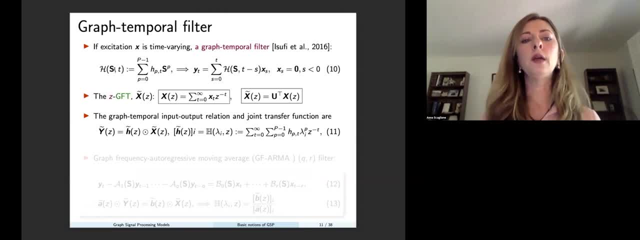 is going to be an operator that here I more conveniently describe as having a dependency both on time and on the GSO, And it's going to be a series of matrix, polynomial for every time t, So that the input-upload relations are going to be consistent. 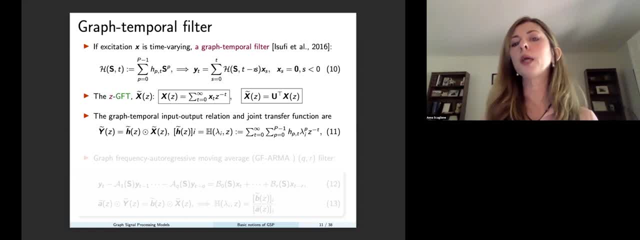 So it's going to be a series of matrix polynomial for every time t, So that the input-upload relationship is essentially a convolution with respect to the index t and is a matrix polynomial multiplication with respect to the GSO. And analogously, when we combine the GFT basis, it might be more convenient and expressive. 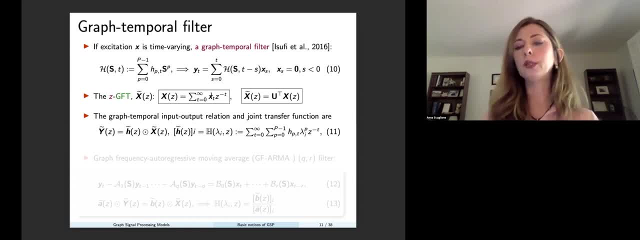 to just look at the Z-transform or the Fourier transform. that will just simply be obtained by replacing Z with e to the j omega And then combining that with the GFT, by taking then the mapping u transpose x of t and obtaining the Z-GFT transform. 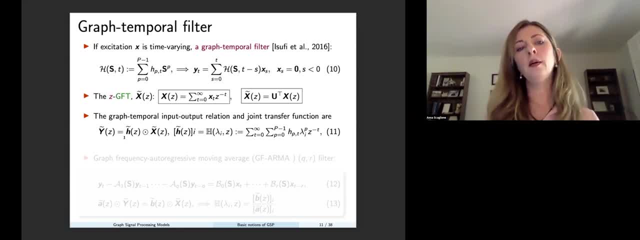 Also in this case, when we take the input-output relationship, equivalent relationship, since in this case h of z is in fact a matrix of value for every lambda i of the graph and every value of z, and then we have an element by element multiplication between these two. 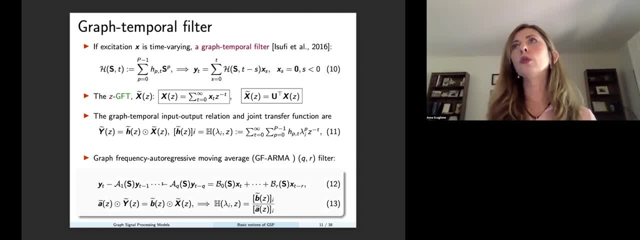 and in this domain you can also define what are called graph, field graph and arma filters, where the ar feedback part is represented by certain matrix polynomials a1, aq of s and instead the ma part, the moving average part, is represented by these matrices and the transfer function in. 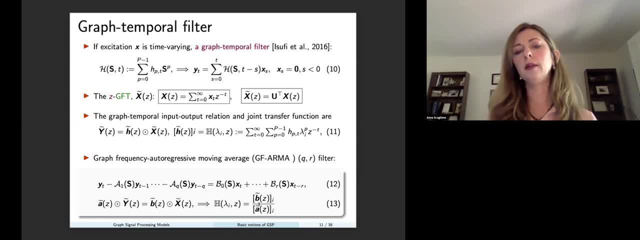 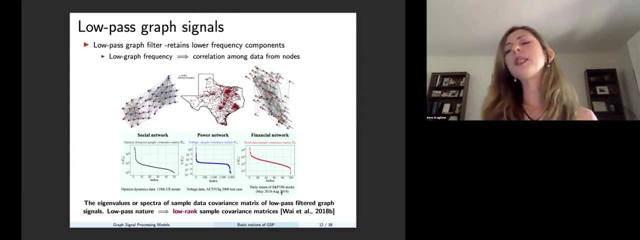 this case can be obtained by dividing the corresponding element of the matrix of the polynomials that are defined in 11 for the b and q matrices. now what's interesting is that power system signals are not completely arbitrary in their structure, because system matrices have certain properties and in particular, they belong to the class of low pass graph signals, which 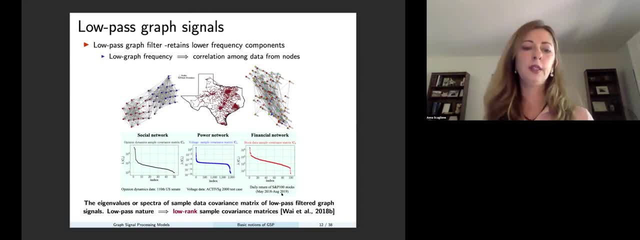 emulate the concept of low pass signals in the in the time domain. so what they do is essentially they retain also especially the low graph frequency components, and this is actually a phenomenon is very frequent for many dynamic assistant model data from social networks to financial networks and the 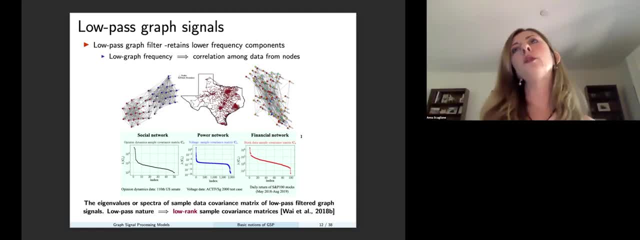 other interesting fact is that that reveals- an observation that has been done empirically studying uh phasor measurement units data- that the data, the voltage phase of data, are inherently raw rank um. so most people are taking principal components from this, but in fact we will see that, since we 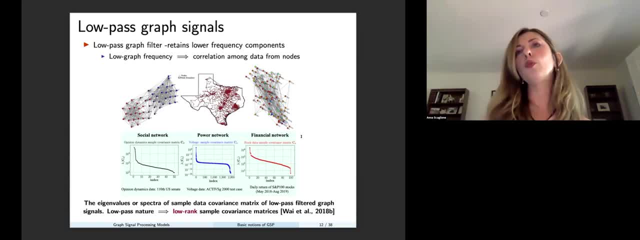 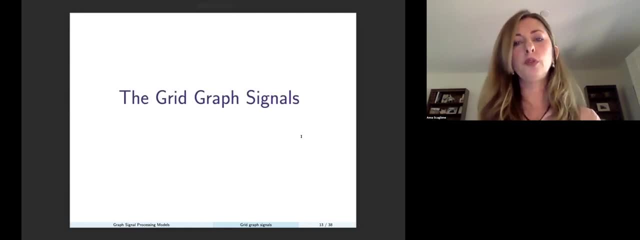 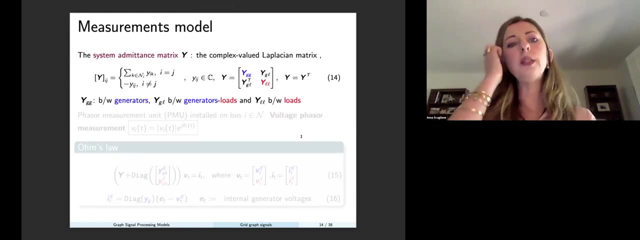 know what is the gft basis based on the system matrix. we actually know what is the subspace ahead of time. so let me then briefly- uh- for this audience this should be trivial- talk about what is the measurement model for phasor measurement units, in particular um, and this is based, obviously, on the electrical laws that characterize the voltage. 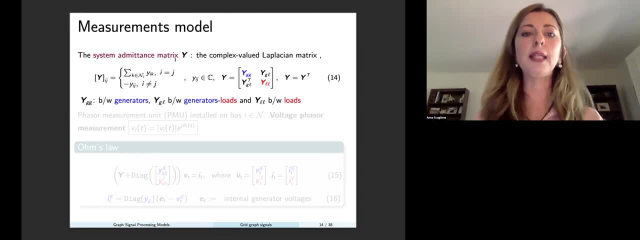 phasors and they depend on the system admittance matrix, which is in fact this complex symmetric laplacian, weighted laplacian, and i'm going to partition these metrics in the: the block that pertains the generator buses, which is this ygg, and the block that pertains the load buses. i know that. 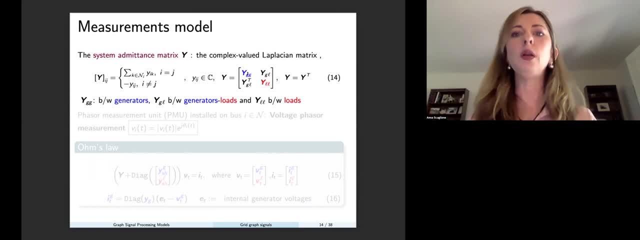 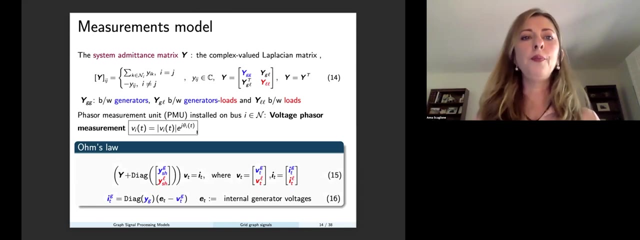 there is typically some overlap. in this case they will belong to the generator buses, class and um, and then obviously there are the blocks that connect generators and loads. and so if we look at the um, fundamental, uh, basic law for the physics of electrical signal, what we we are writing is: 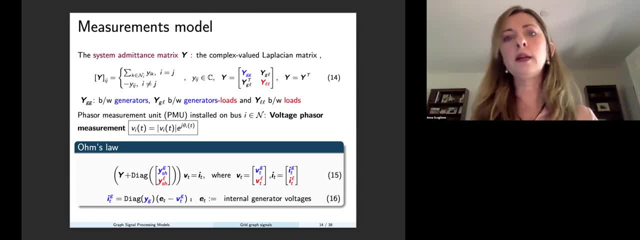 holmes law, where the relationship between current and voltage is characterized by the system matrix plus a matrix with the so-called shunt elements for generator buses and load buses, but what is also important, particularly for the development of the time dynamics in the sort of graph signal. 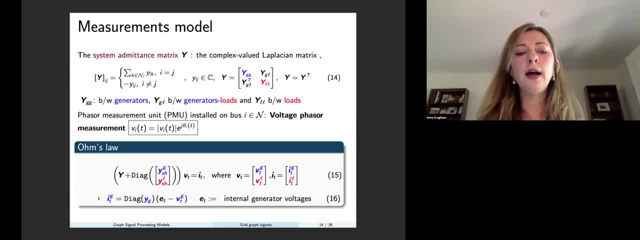 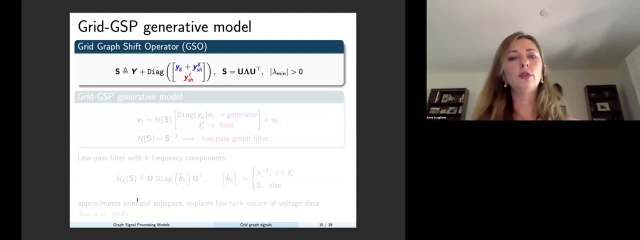 processing perspective is to explicitly express the current of generators as a function of the so-called internal generator voltages, and which are called ET, and instead YG are internal generator admittances. So what is the grid GSP generative model? It is obtained by assuming that in fact, 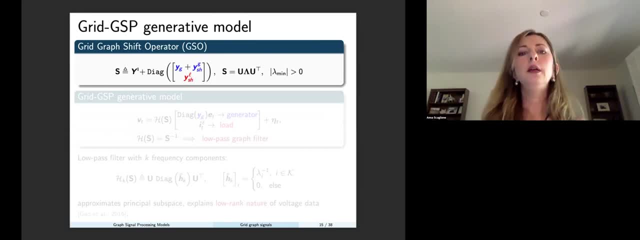 the graph shift operator is nothing but the matrix that we saw here, augmented with the generator buses admittances. so it's y plus the diagonal of the YG, plus the Y shunt for the generator buses and the shunts for the loads. and if we take the GFT of 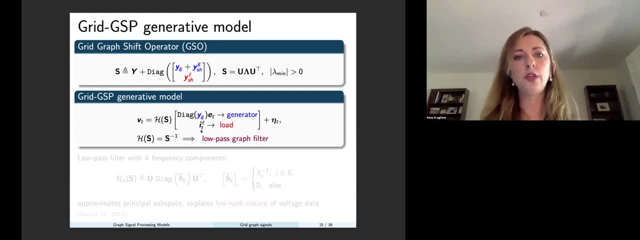 this, then we obtain the correct GFT basis. sorry, if we take the eigenvalue decomposition of S, we obtain the correct GFT basis for electrical signals. and the input output relationship is actually quite simple. it states that the voltage is equal to this graph filter, which is very simple. 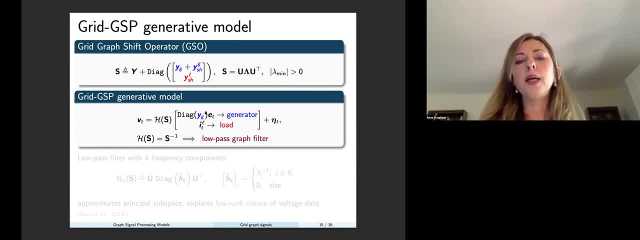 it's S to the minus one multiplied by this excitation, one that depends on the generator buses, internal voltages, and the other one which is the current of the loads, and this is the classic integrator. if you interpret S as the S in the Laplace, transform one over S, we know is the integrator. so that's exactly the effect. 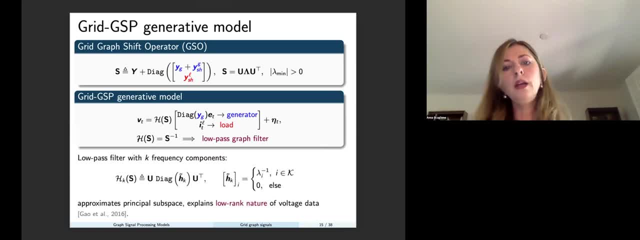 of the system matrix and if we just look at the what happens in the frequency domain, we can see that it could be these graphics that could be easily approximated with a system that only has k frequency components and, in particular, transfer function would be one over lambda i, over the subset k and while other elements can be zeroed out. why? because 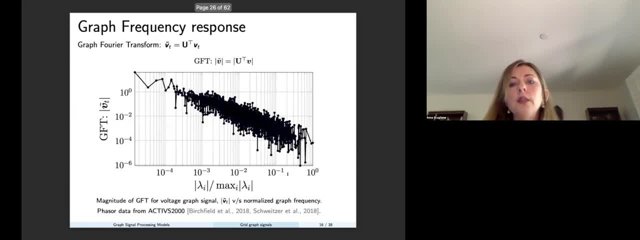 because essentially the lambda values for a typical system matrix decay, very decay, very rapid ly, or vice versa. in this case one over lambda increases very rapidly as lambda approaches zero. so this is the exam, an example of the GFT, of synthetic phase of measurement data from the 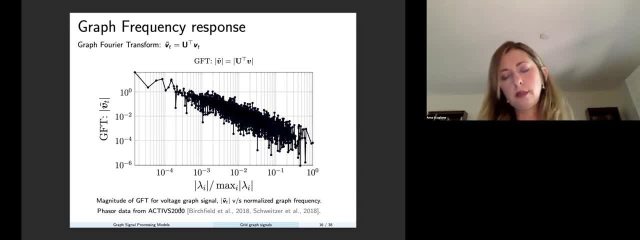 actives 2000 synthetic case that emulates the Texas power grid versus the normalized graph frequency, so the eigenvalues of the GSO, and you can see that in log scale. clearly there is a very rapid decay in the spectrum of the voltages. that is simply interpreted. 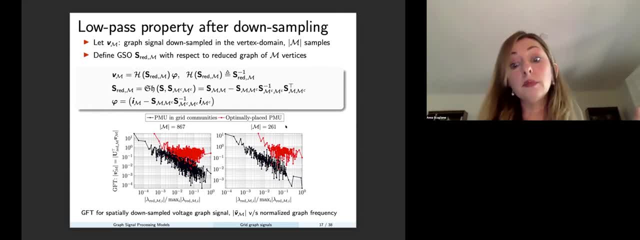 as i mentioned before, due to the fact that the system equations are essentially an integrator. not only that, but also that the typically the, the GSO, is highly ill-conditioned. the other interesting factoid is that, even if you don't find yourself with a complete set of 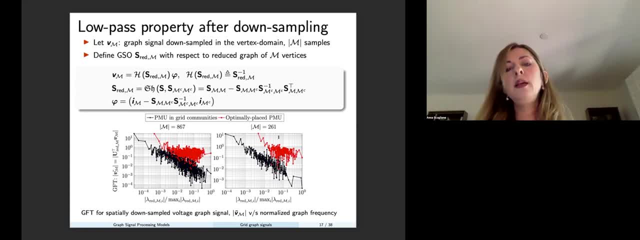 PMU data for the system that you want to analyze. any decimated graph signal is also a graph signal. obviously the GSO has to be modified. in particular, we need to take the sure complement of the matrix. correspond to blocking the GSO in the part that pertains the measurement set. 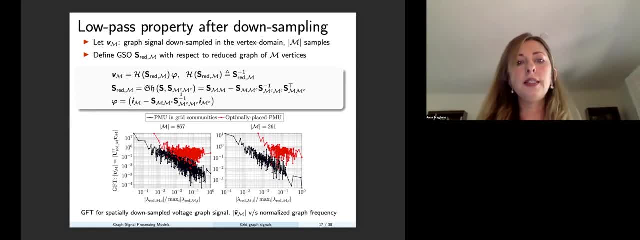 and the part that pertains the complementary set and the excitation in this case not only contains, obviously, the input current for the measurement set, but also has a component that comes from the currents that are not measured. that we can interpret, though, as noise added to the signal. 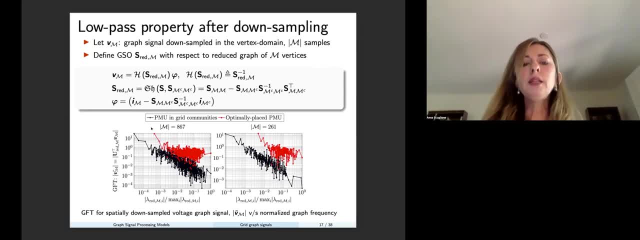 and the more you decimate- not surprisingly- the less pronounced is the low pass behavior of the signal. nonetheless, you can see in the pictures that the red GFT for a decimated set- 860, 7 buses out of 2000 or 261 buses out of 2000. you can see that the red line is still decaying. 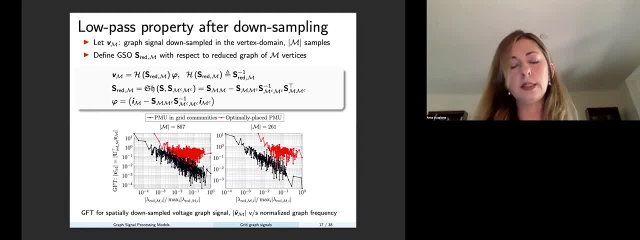 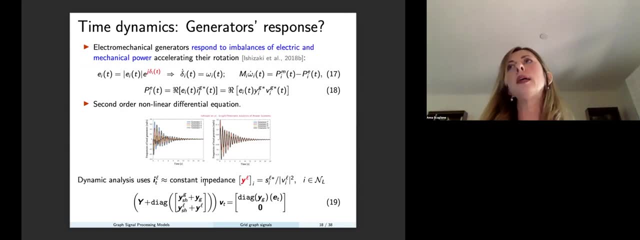 even though the original line is decaying much faster for the complete system. so what about the time dynamics? the time dynamics are should be based again, just like the spatial properties, on the physics of the system, and what we know is and what we can leverage in this case are the 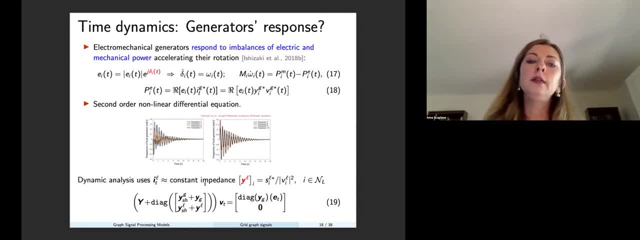 the swing equations that express the dynamics of the angle of generators, buses of the generators, and they express them obviously as a function of the imbalance between electrical and mechanical power and that would allow essentially to provide dynamics for EOT. but it's important to notice that obviously there is an immediate relationship between the phase angles of the generators. 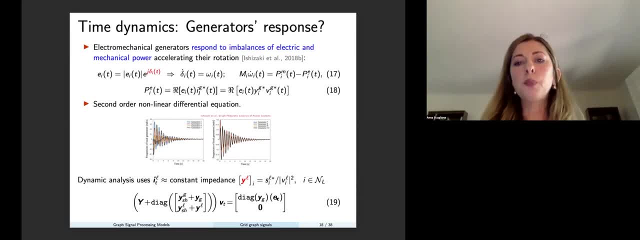 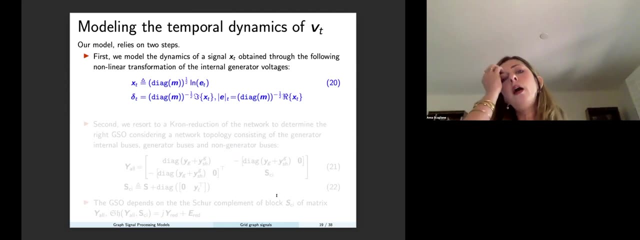 and the signal that we have here. so, as you would expect, we cannot express the GFT model completely as a spatial temporal process over the product graph, but there is a non-linearity in between. and, in particular, what we can do is we can define a GFT model, a GFT temporal model, for the generator bus only network, but we need to first of all. 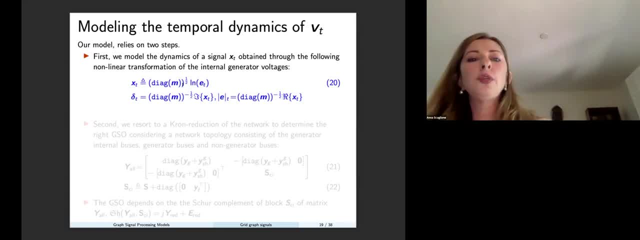 rescale by the square root of the masses. each of the entries of a vector that contains the logarithm of the internal generator voltages, which means that the angles are going to be the imaginary parts of this vector, while the real part, the magnitude, will be the other component. 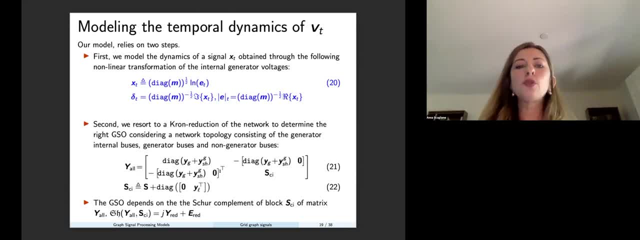 to capture, and the way we obtain a GSO for this model, obtain taking this normalization and logarithm, is by converting the loads into constant impedance loads, as it is done normally in analyzing the dynamics of generators, and once again taking the Schur complement of the overall matrix. 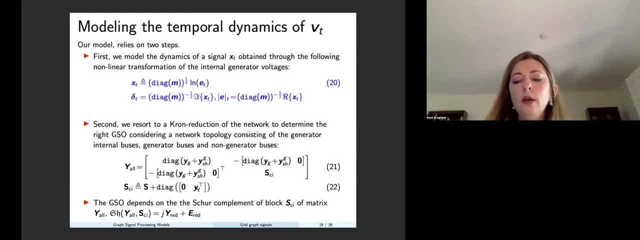 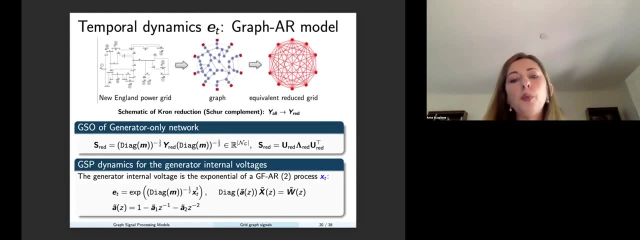 where we added to the block that correspond to the loads, the equivalent admittance and with Schur complement, what we can obtain is a graph temporal filter with GSO which is equal to this current reduction of the general only net of the original network, rescaled again by the masses, and with that we can prove for the, for the angle, that 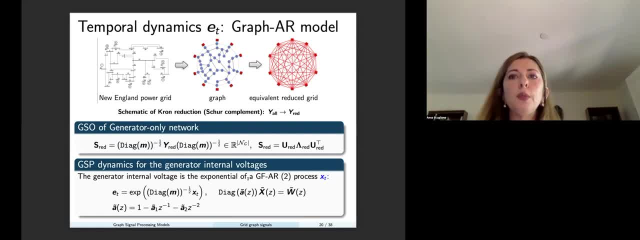 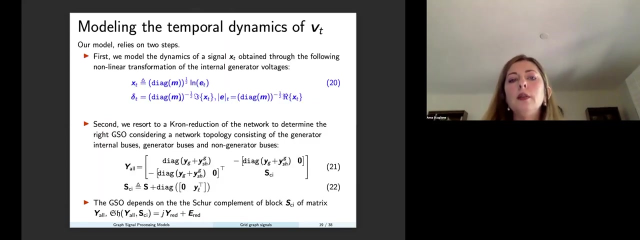 in discrete time. the second order swing equations can be approximated unsurprisingly by a second order graph AR filter, and the heuristic that we applied- the model we see in the moment works very well- is to also assume that the logarithm of the amplitudes of the generator buses follow a similar process. so our description is only next. that contains both. 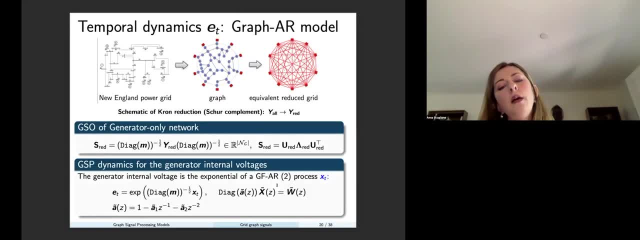 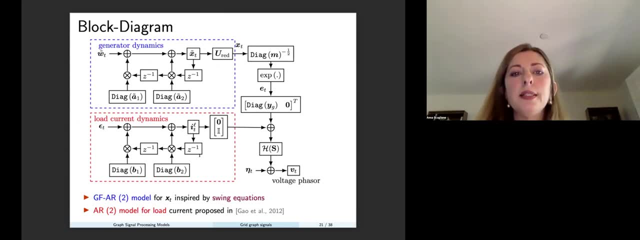 the, as imaginary part, the angles, and as a real part, the absolute values, the logarithm of the absolute values. so these kind of summarize the model that we have, the, the model we have for this spatial temporal structure of voltage phasors, the generator dynamics. are these second order graph filter, AR model. where you read is the: 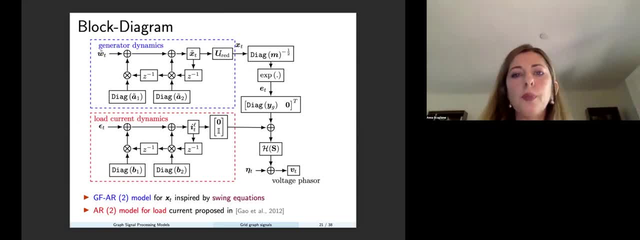 GFT basis for the current reduction for the particular GSO that I showed here. then we, just as I said, rescale by the masses and then take this exponential operation to get the generator buses load. then we reweight this by the generator admit admittance and the current dynamic we also can model as an AR2 model. this is just an empirical. 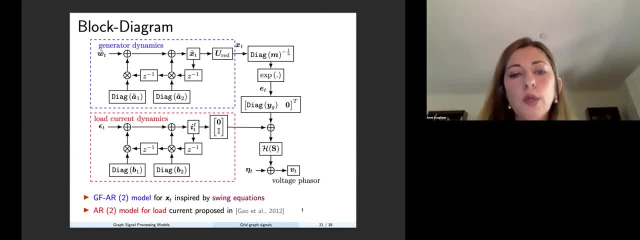 observation taken out of this paper by Gao in 2012, where they show that this is a reasonable model to capture the in the dynamics of the load current. and all of this goes through the graph filter we decide, we described for the entire voltage, which is, as we said, simply s to the minus. 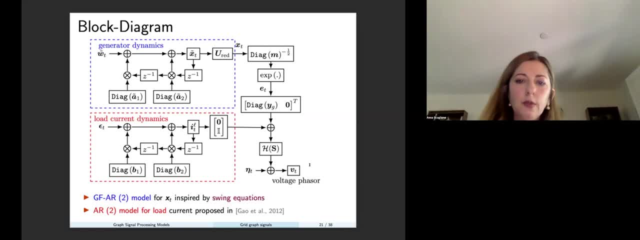 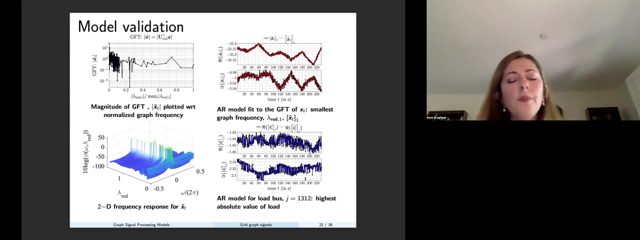 one where s is simply the system matrix, with the additional shunt elements and internal generator graph generator admittances, and then obviously here we say that it just represents a modeling error that is obviously also associated to these dynamics and this, essentially, is the entire generating model for the voltage phasors. and the fact- and here what we do is we validate- 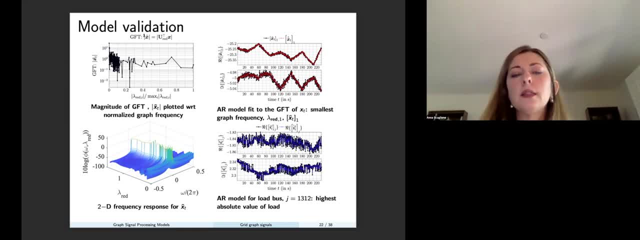 the model for the dynamics of this signal x, which is the logarithm, the rescale logarithm of the internal generator buses. this is the, the spectrum that we obtain for the signal s in the graph frequencies, and versus omega in time, and you can see in the red and black curves that the tracking 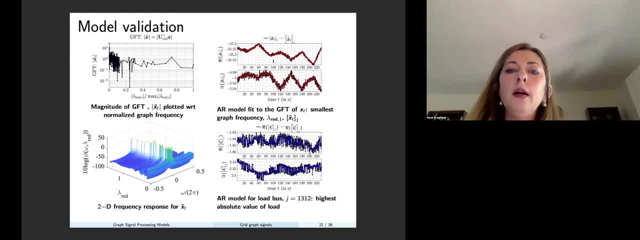 of the real imaginary parts of the signal x are quite accurate if we look at the gft of them and look at the evolution in time. so this is essentially what the model says, how it tracks the signal versus in in red and blue, versus what the actual signal is. 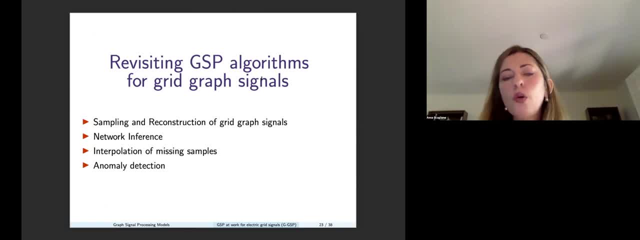 in black. so, now that we have introduced all this modeling, this mapping, what can we do? certain things are absolutely straightforward. right, so we know that the signal is not a linear model. right, and then we know that the signal is not a linear model. so we know that the signal is not a linear model. 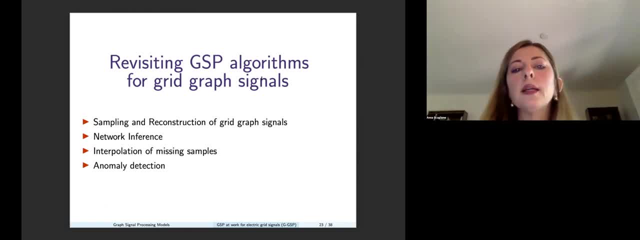 So, just like DSP for GSP, there are sampling and reconstruction theorems. There are algorithms for network inference, however, that are not necessary. in DSP. where we actually know the underlying graph, We can relate it to. sampling also is the idea of interpolating missing samples. 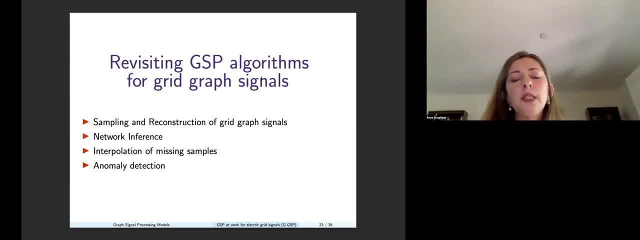 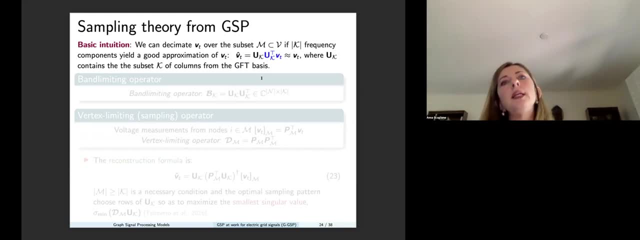 We can perform anomaly detection and also relate it to sampling and reconstruction is the idea of compression. So let me talk about the sampling theorem and how is sampling related with the problems that appear on the grid is, essentially, how do you place your sensor? So that's a sampling problem of this irregular support. 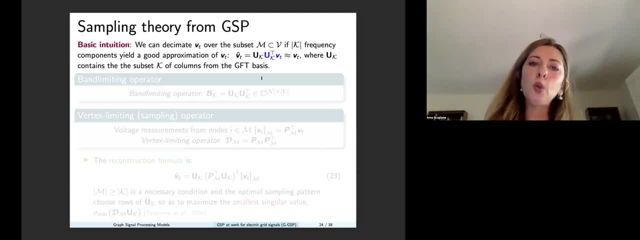 And the basic intuition is that if the support of our graph signal is sparse in the GFT domain and in particular we know of our systems- we said it's low pass- Then what we can do is We can construct an approximation of the original signal V of T by projecting it only on this most significant frequency component, as I said, the low frequency component for the power signal. 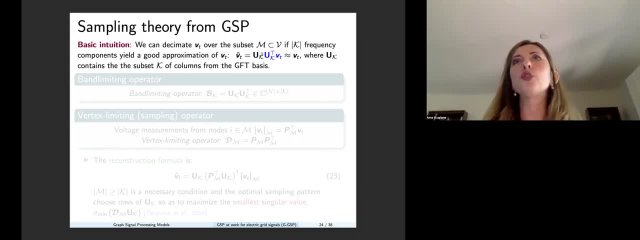 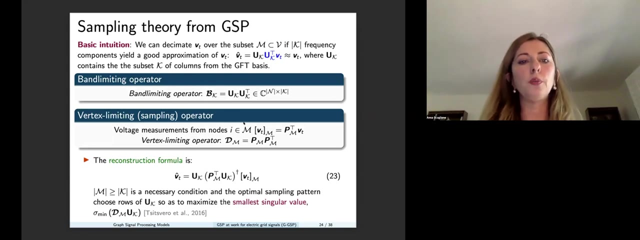 And then obtain an approximation by essentially projecting back the signal over the original complex space, And what this essentially represents is the equivalent of an anti-aliasing filter and it's called the band limiting operator. It's essentially a projection, While sampling can be called vertex limiting operator. it's just selecting only some vertices and selecting a particular vector of samples out of the original. 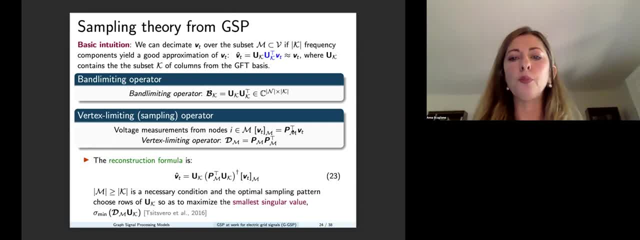 phasor. So this can be expressed with this selection matrix P of M And the reconstruction formula that can be obtained with simple algebra. If you have a matrix, this matrix, which is the matrix of the original phasor, which is the selection operator, times the subset of frequencies that are most significant, if this matrix is invertible, then the reconstruction from sampling is performed in this fashion. 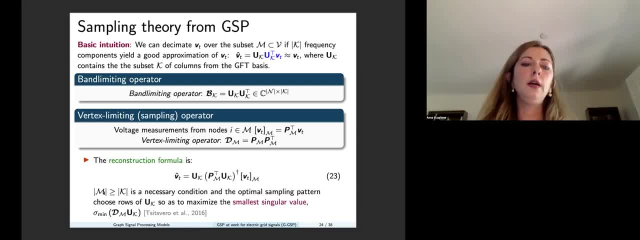 And obviously the fact that you have more measurements and the frequencies that are utilized is a necessary condition for that. But how do we obtain a sampling pattern which is optimum? We can simply try to minimize a proxy for the good invertibility. So we can simply try to minimize a proxy for the good invertibility. 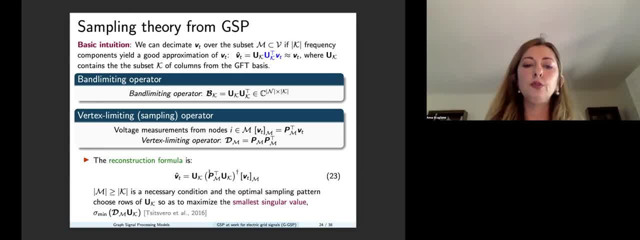 So we can simply try to minimize a proxy for the good invertibility. We can simply try to minimize a proxy for the good invertibility properties of the operator here that you see in Legation 23, which amounts to maximizing at least the minimum eigenvector of this matrix. 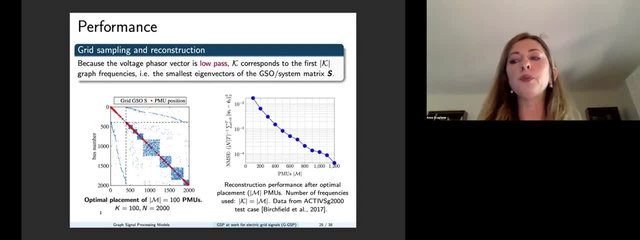 So let me show you the performance of this optimum sampling. now, obviously optimum search for a support is a combinatorial problem, But greedy algorithms return a fairly good solution and the information we get from this is very, very good solutions. Here I'm showing on the left-hand side the SPI diagram for, again, the ACTIVS 2000 cases. 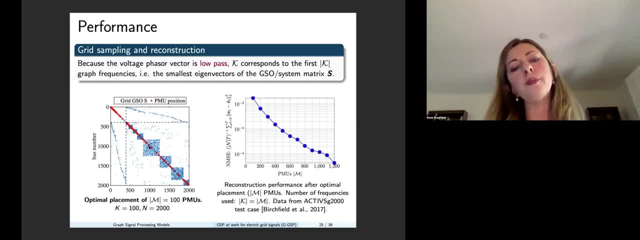 2000 bus system emulated in Texas. You can see that the graph presents clear clusters. These would be the major cities in Texas and they tend to be connected to different generators. Now the reconstruction performance are actually quite outstanding. You can see that. 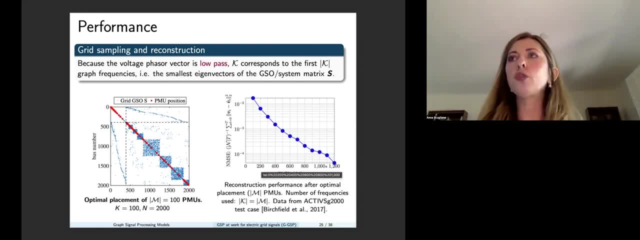 only utilizing 200 phasor measurement units you will be able to obtain an error percent, an error which is just one percent of the pair measurement. and these curves deeply decreases as you increase the number of measurements. So it's an order of magnitude. 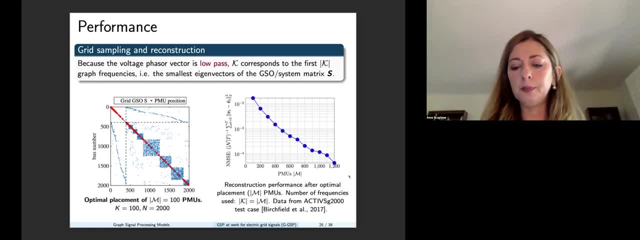 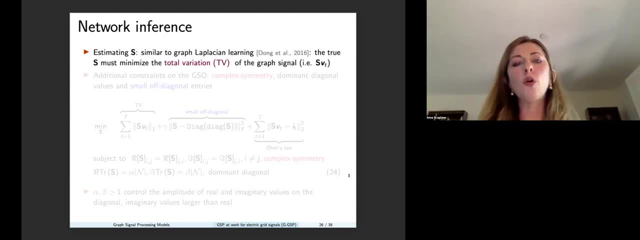 lower number of measurements than that Number of passes So well below observabilities. Network inference is also a problem that can be formulated Now. keep in mind that many people have utilized graphical lasso, which is the typical method to identify the structure of a graphical model. Bayesian graphical model. 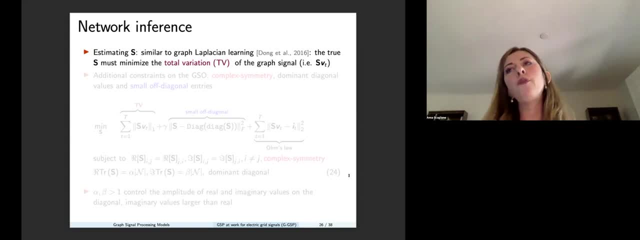 to the problem of network inference. The beauty of relying on the physics is that you can incorporate more constraints, which are physical constraints, but in addition, you can interpret the idea of graph signal processing to provide you other terms in the objective, such as minimizing the total variation of the signal, now with respect not to V, but in this. 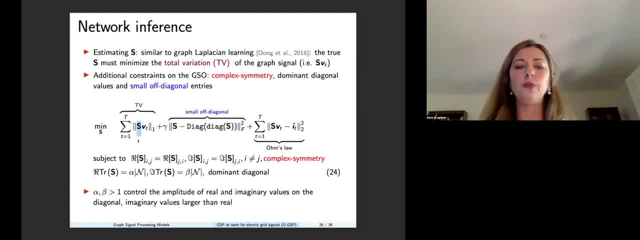 case with respect to the GSO itself, which is the objective, the argument of these, disoptimization in the network, inference problem, And you can add a number of other constraints like you want, a small off-diagonal terms just to enforce sparsity. 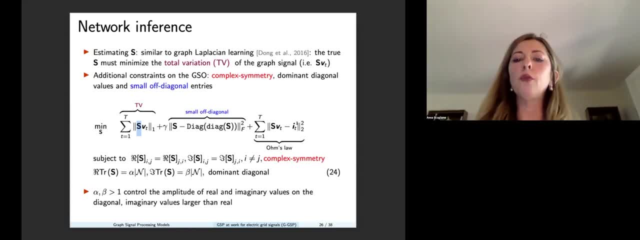 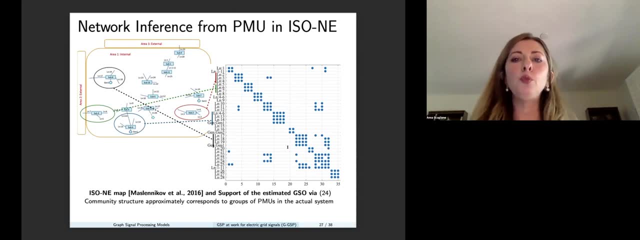 and a small non-form of diagonal terms, And obviously you can also introduce Ohm's law, And here it's an example. finally, on actually real PMU data from ISO New England. As I said, if you decimate you can still have a low-pass graph signal. 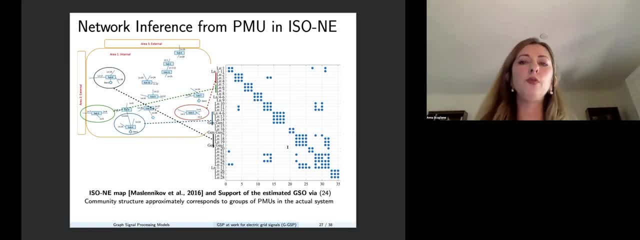 So the properties that we want are satisfied, even though we don't have, obviously, a complete set of measurements for the ISO New England. And you can see that the algorithm I just presented, the minimization, provides an inference on the topology which is very similar to what is represented in this graph. 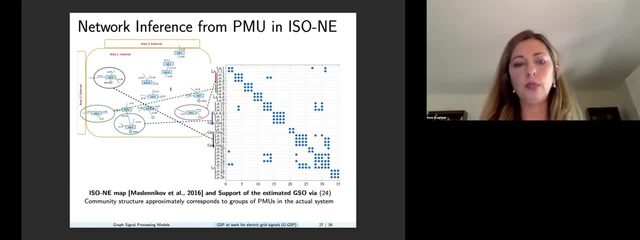 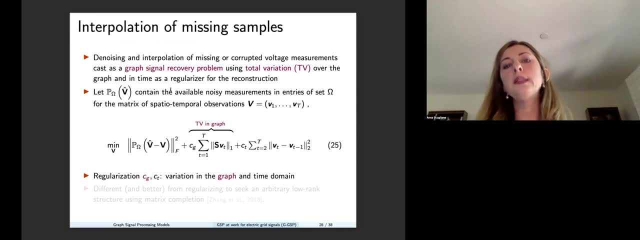 that is given along with the data for the ISO New England. The same idea that you have a low-pass signal can be utilized to interpolate missing samples, And the key point here is that you know what are the dominant frequencies. So, again, you utilize this in a regularizer. 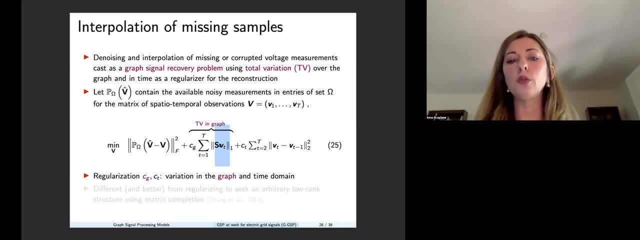 that tries to minimize the total variation of the voltage that is reconstructed And in this case not all measurements are missing. So if the measurements are B hat, you're gonna make sure that the set of phasors that you reconstruct minimizes the distance. 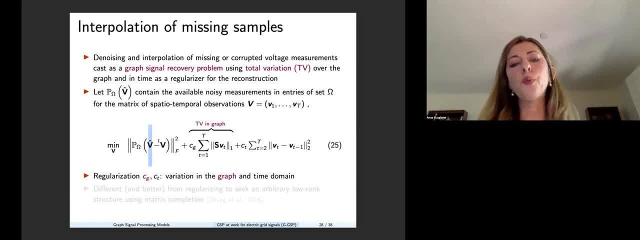 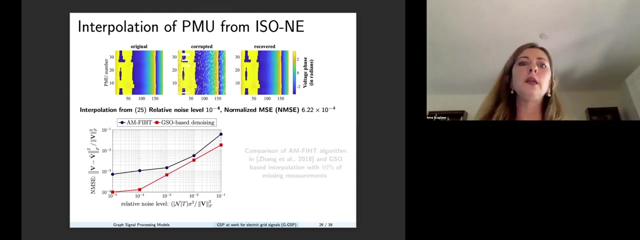 between the measured values. So with a certain support with the true values, And since we also know that the dynamics of the voltage phasors are slow in general time, then we can also utilize as a regularizer the variation in time. Now the idea of interpolating missing measurements. 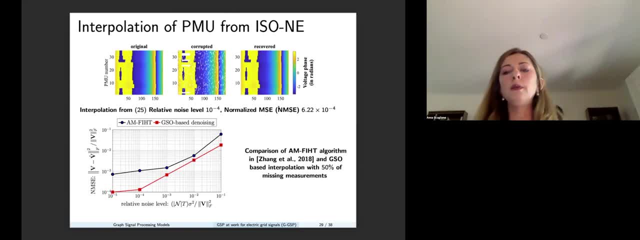 is not new. There has been interesting work by Zhang in 2018 that applied a matrix of the and the of the voltage phasors. So here you can see the ISO New England segment of this data, which is synthetically corrupted as shown in this figure. 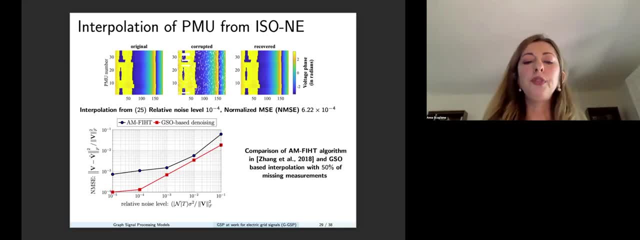 And the recover signal is on the right hand side. So you can see that the result based denoising of these data performs better than the algorithm proposed by Zhang in 2018 and co-authors. And the simple reason is that, instead of using 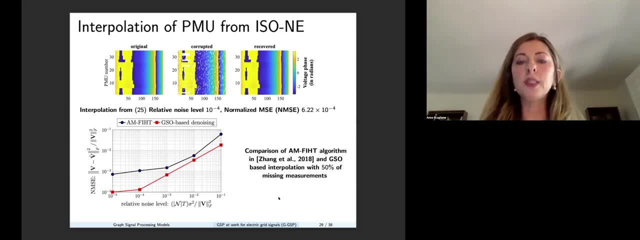 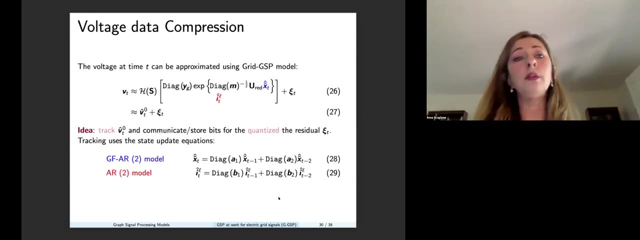 as a regularizer is the fact that the measurements need to lie in a low dimensional space. we actually know what is the low dimensional space, We know the GSO and so we perform better. The other natural takeaway message: if you have a model that allows you to show that there are components, 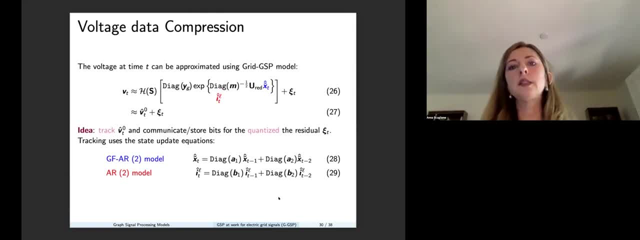 of the signal in a certain domain that are prevalent and others that are very small, is to utilize it for data compression, And in particular here. what we want to do is to say that from previous samples, previous compressed samples, we can essentially estimate, track. what is the voltage? 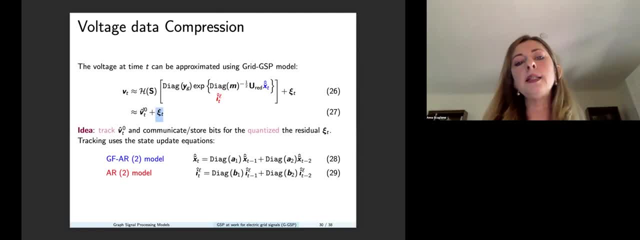 And obviously there is a residual error, And the idea is that this part, this V naught of T, can be obtained, as I said, from the previous sample without transmitting additional bits. So the task at hand is just truly only compressing these residual. and since these residual is again sparse, 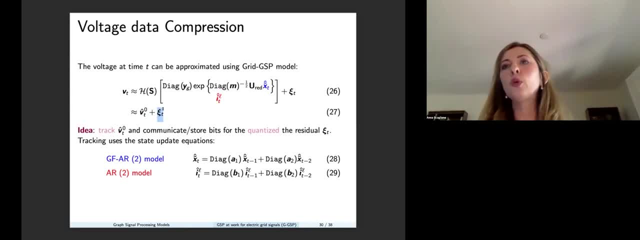 in the GFT domain, what we can do is bit loading, So loading more bits in the high components and less bits in the slow components. And how about this? How do we track? V naught, We utilize the ARG graph filter, AR models for the dynamics. 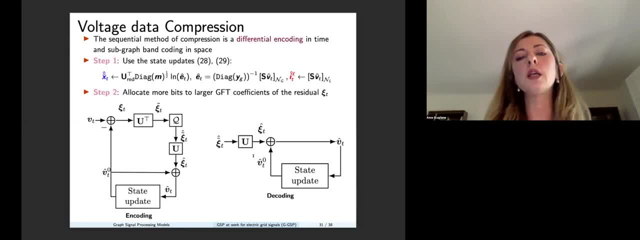 of generators, of the logarithm of the generator voltages and for the load currents, And so this is the block diagram of the scheme. So the step one is we take past value to track and estimate the GFT of the logarithm of the generator buses. 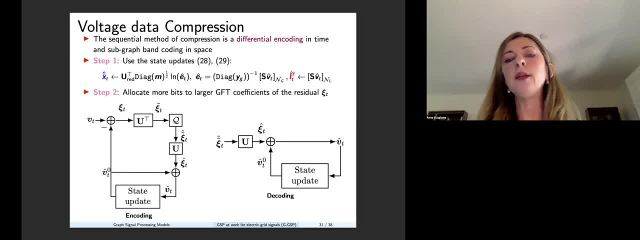 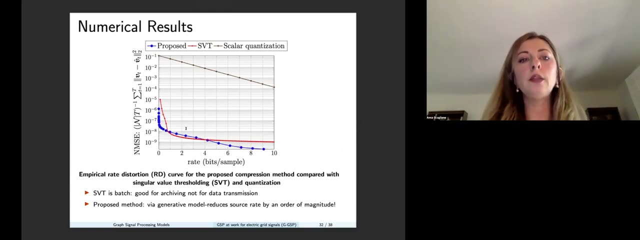 internal voltages and of the load. And the step two is we utilize the bits that encode the residual to reconstruct the next sample. The numerical results are state of the art. This is the blue line that shows the distortion on the reconstructed voltage versus the number of bits. 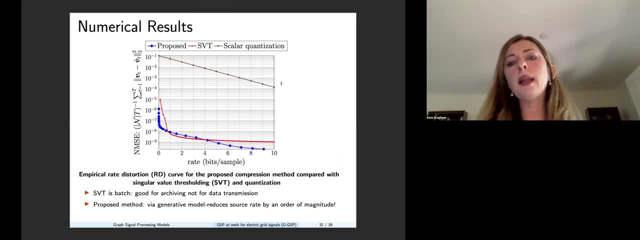 that are assigned per sample. The black line is what you would obtain if you just simply do scalar quantization, And the red line is what is considered state of the art, where you take an SVD of the data and then you essentially prune the SVD from the components. 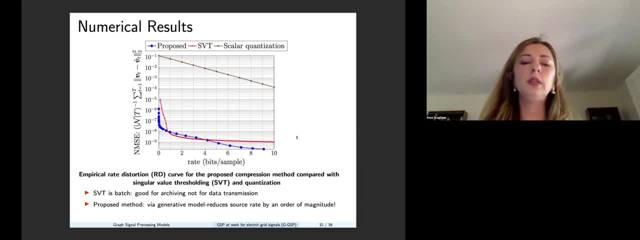 that have the smallest singular values and just encode the components that correspond to the higher singular values. Now the notable difference is not only that our curve doesn't saturate, but also that we have a sequential scheme. So this cannot be used Both for storage of data but also for transmission of data. 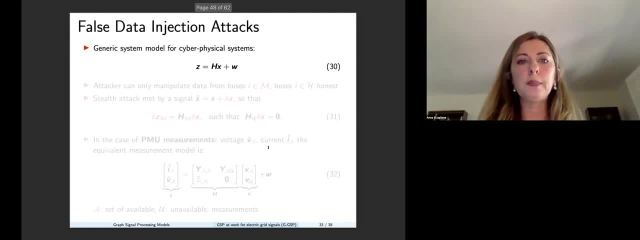 this allows to transmit sequentially with a minimum number of bits. Let me go to a security problem, since this is the theme of this particular workshop seminars. So false data injection attack is a beloved topic where there are a lot of contributions in the literature. 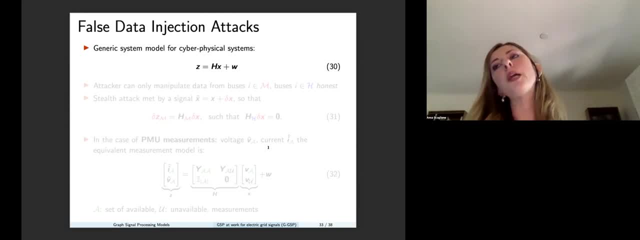 But once again, my point is that the GST framework sort of naturally leads to an excellent algorithm to detect such attacks. So let me explain briefly, for those of you that have not stumbled in papers on this subject, what is the mechanic of the so-called stealth attack. 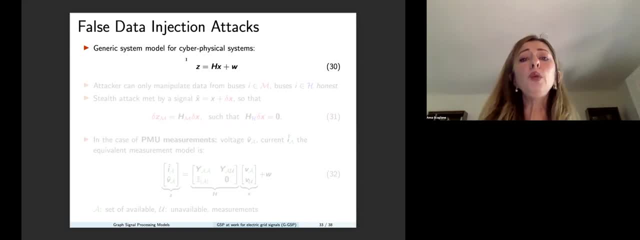 to cyber-physical system. So we have system equations that model our observation z And they are linear. They are linear And in this case obviously there are measurements, So we have some noise. So the premise is: the attacker can only. 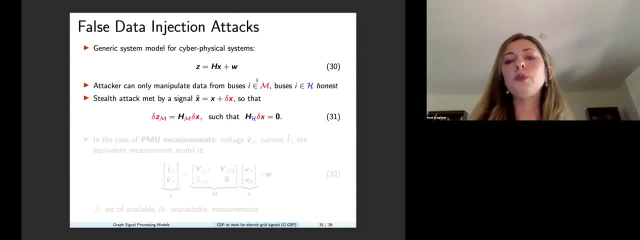 manipulate a certain subset of the measurements which we call m And there are h honest nodes. So how do you design a stealth attack? You design a perturbation which has the same sparsity as the number of measurements that are controlled, that the measurement set is controlled. 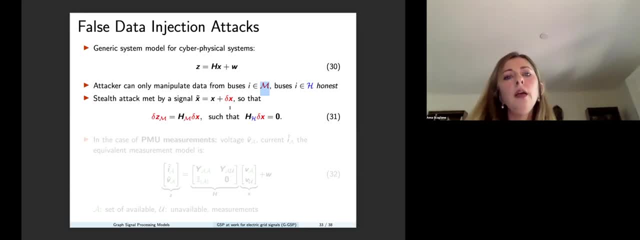 by the malicious agent, Such that this will actually introduce a non-trivial perturbation of the observation vector. But at the same time, these sparse vector, if is multiplied by the rows of the system that correspond to available measurements, these will give zero. 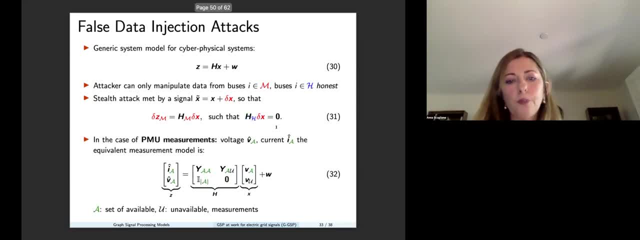 So, in other words, this is in the null space of this operator. In the case of PMU measurements, h is this matrix, which is the admittance matrix of the NER Available measurements, and the admittance metrics here is the one between available and unavailable measurements, and Z is this observation. 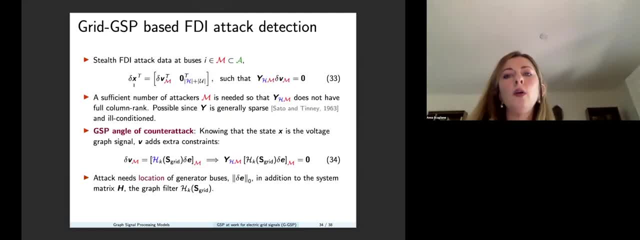 So how does the attack work in this case? Well, what matters is that the perturbation of the voltage phase of measurements has to lie in the null space of the block that is up there, which is, in the case of the malicious attack, the block that connects the 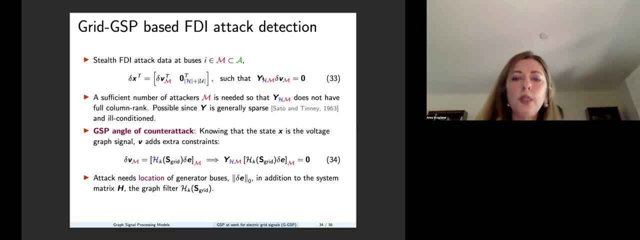 Honest points, like the points that are not attacked, with the points that are attacked. Now, how does the GPS angle allow us to study this, A counter attack, in other words, to detect these attacks? because we know that we can rely on the graph signal processing model and, in particular, proximate the measurements as something that lies in the subspace, which is the subspace that is highlighted by the graph filter. 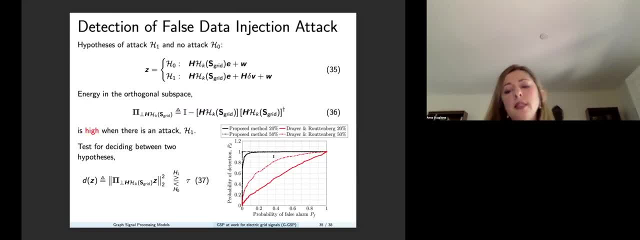 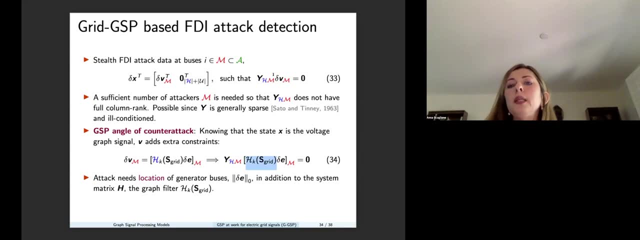 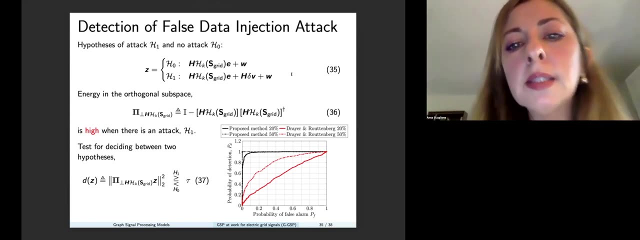 And so this essentially constraints significantly what should be the structure of the graph Of the attacker, And so this becomes quickly incompatible. You have too many equations with respect to these constraints for the stealth attack. So the type of hypothesis test that can be formulated is, in the case of the null hypothesis, is that you have something that respects the 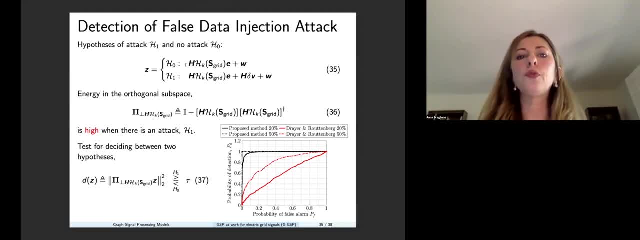 Normal Equations for the represented GSP model, the complete GSP model. instead for the Modified hypothesis, you need to have this additional component. What these additional component does is introduces More energy, so to speak, a larger contribution to the frequencies that are instead suppressed by this graph filter. 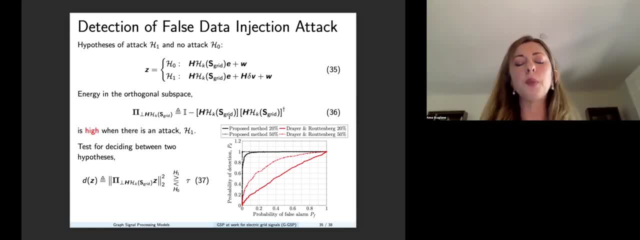 So if you utilize an orthogonal projector to the subspace, we can have this very simple metric Which states the norm of the projection of the observation vector on to this orthogonal subspace And if this norm exceeds the threshold, so if there are high frequency components that 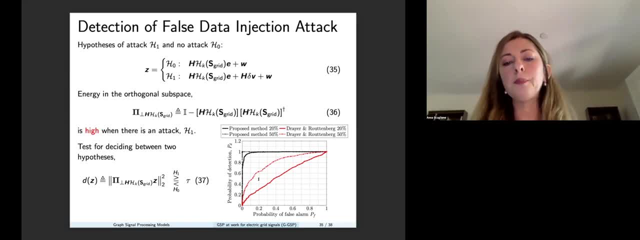 shouldn't be there. then we detect a fossilized injection attack. So here there is again a comparison. Our method is in black, A competing method is in red. You can see that even if the agent has a large number of available attacked points, 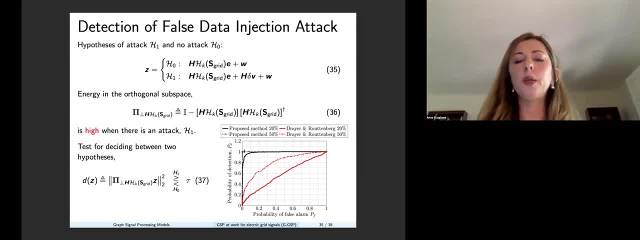 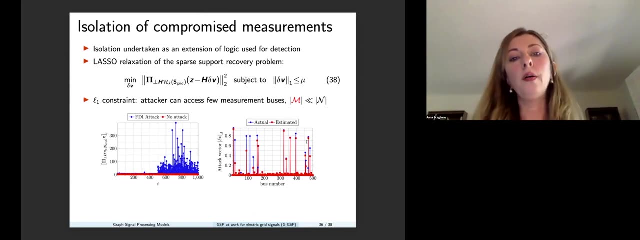 then our performance in terms of the receiver over any characteristics- the probability of detection versus probability- is very good. It's this black line. The competing method doesn't perform as well And in the same spirit, we can also have a reasonable estimate. 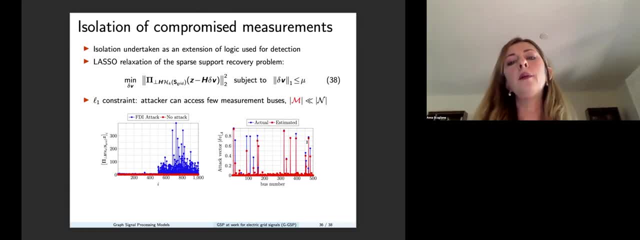 Of what are the measurements that attack? essentially, by saying that we are seeking a solution which is sparse, because the attacker cannot obviously attack all the measurements in our model, and trying to minimize once again the same metric that we had before, where we subtract, in this case, 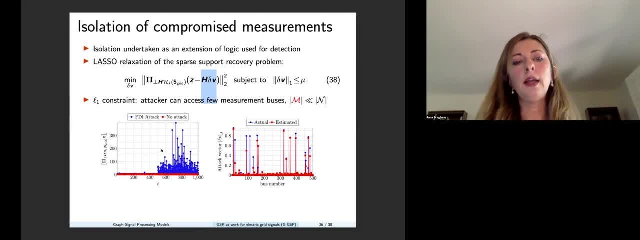 the attack that we are trying to estimate. And here you can see that If there is no attack, then it's clear that all these projections of z on the projector that we described in the previous equation, in the previous slide, gives the result in red. 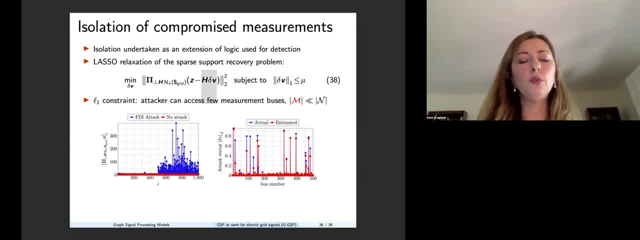 So it's very flat: There is no big contribution there. When there is a stealth attack. instead, in blue, you can see that there is a high contribution here And, exploiting this fact, we can actually relatively well estimate the support. The true support is in blue. 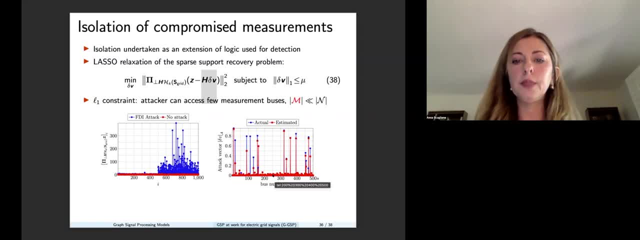 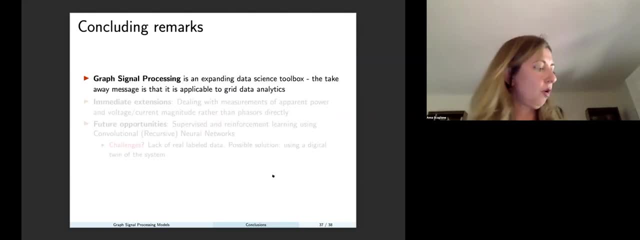 And the actual support, like the measurements that are attacked. according to our estimation problem is 38 of the red, So I am well on time. So, just to conclude, this is scratching the surface and it's just touching the tip of the iceberg. 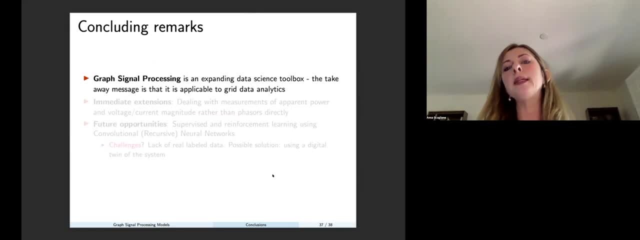 Why? Because graph signal processing is actually an expanding generic data science toolbox, And so the takeaway message of this talk is that you can actually apply it to grid data analytics kind of straight out of the bat, these algorithms that are developed by machine learning and data scientists. 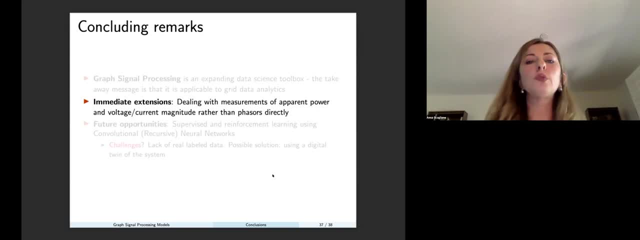 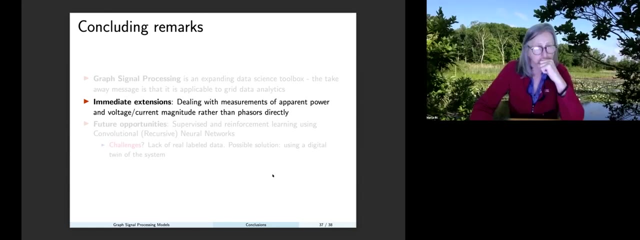 Now the immediate extension is obviously dealing not just with phasor measurements but also with power flow measurements and in general power, apparent power measurements and voltage and current measurements, And here obviously the connection to GSP is indirect. 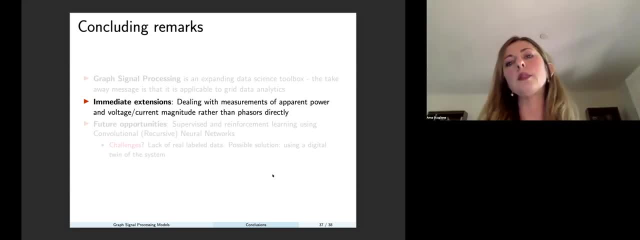 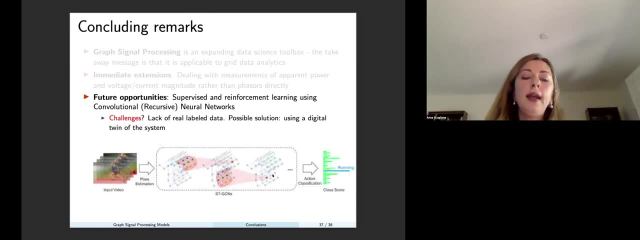 But there are a lot of opportunities to utilize this model and capture the features of this data, And the future opportunity in purely the machine learning area are extending, also something that has become a very interesting area of development in video analysis And also image analysis, which it 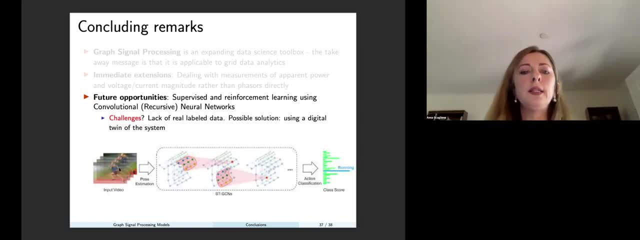 is to associate a graph to the interesting parts of an image and track essentially the sorry and view the image itself as a graph signal. And for this case, what is a better parallel is with video analysis, because we have in the grid, as we said, the spatial temporal process. 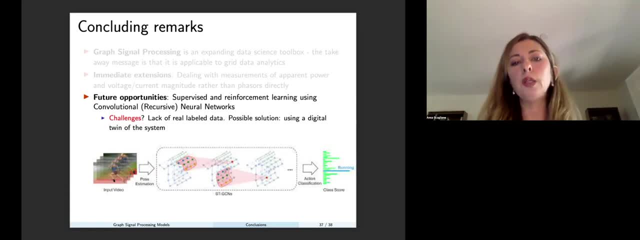 And so there is a very interesting set of development in the field. So graph convolutional neural network, And in this case we will use graph convolutional recursive neural networks. And why is this important? Because that becomes an architecture just like convolutional neural networks. 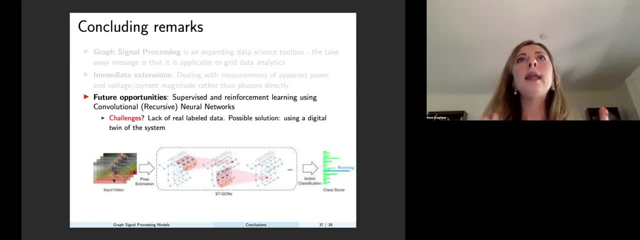 or recursive neural networks that can have in the first layer essentially a feature extraction capability, which is the reason why convolutional neural network and recursive neural network have been So successful. And with that I conclude my talk. Thank you very much, Anna. 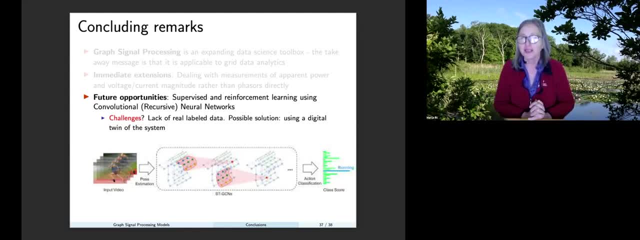 It was a really nice tour through signal processing and to graph theory and what is effectively state of the art in graph theory, And I think we can have just a couple of questions here and then we can move to panel to more detailed discussions. We have a question from Mr Daddy. 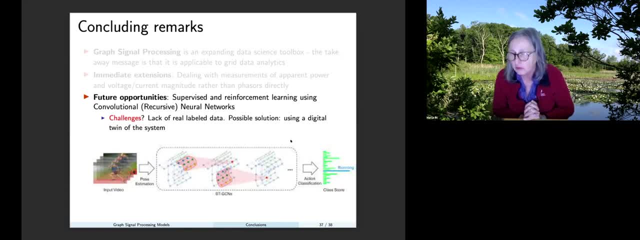 He says: This is a nice talk, This new way of looking at graph theory. Do we get system level time series, repetitive dynamics? That's question one. There are several questions, So let's read one and then discuss that one and we'll move next. 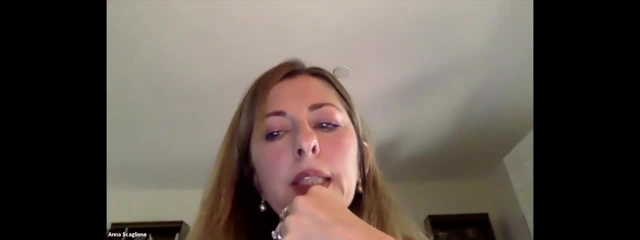 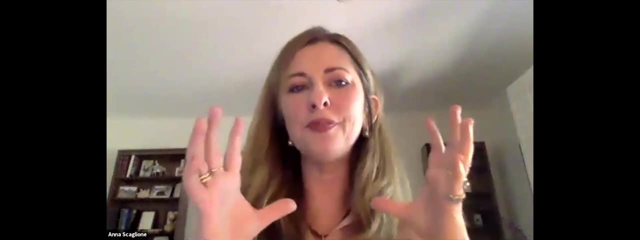 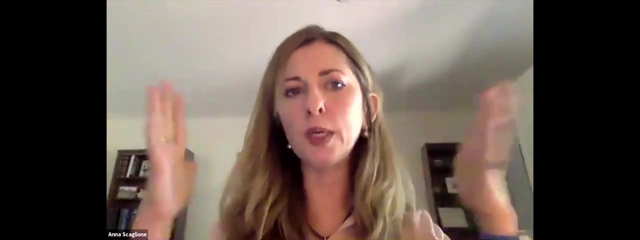 Do we get the system level time series? repetitive dynamics? Not really So. the idea of the cyclic graph? I guess it's a little bit confusing, right? So that's the way DFT develops, the DSP develops the DFT, And typically what you do is you analyze over segments of data. 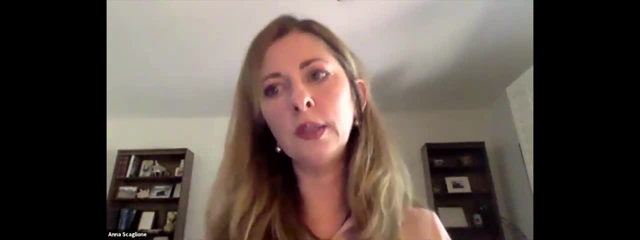 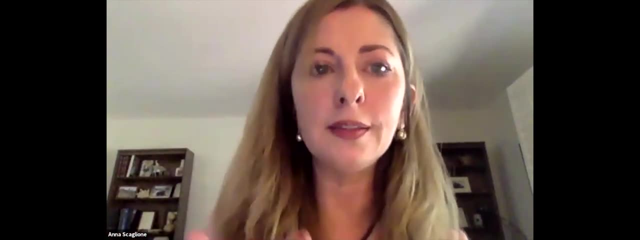 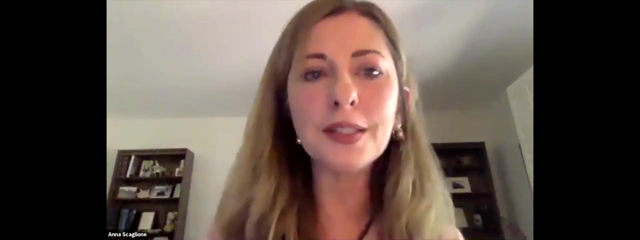 And the DFT is just really a tool to have a corresponding numerical way of calculating a Fourier transform without calculating the discrete Fourier transform which would be over a continuous support. So you don't have to worry about the cyclic graph because we always apply AR modeling and Z-transform and DFT. 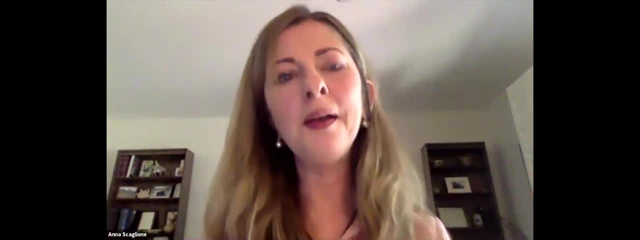 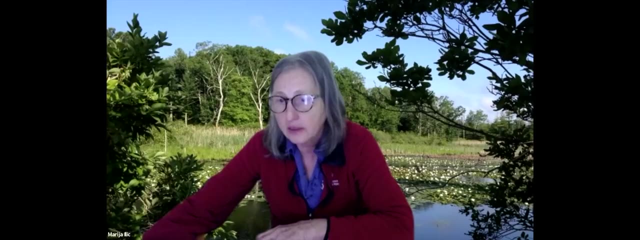 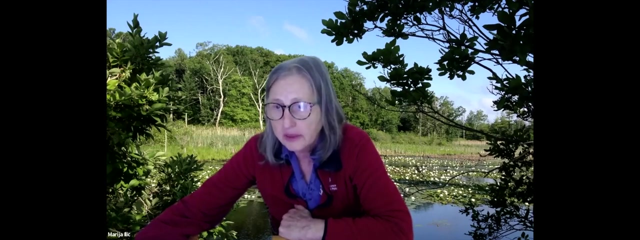 analysis to signal. They in fact are not periodic, But the basic idea is that you analyze them on a segment by segment basis. OK, thank you. The second part of the question is: is it possible to separate system level noise from corrupted data with this new signal processing? 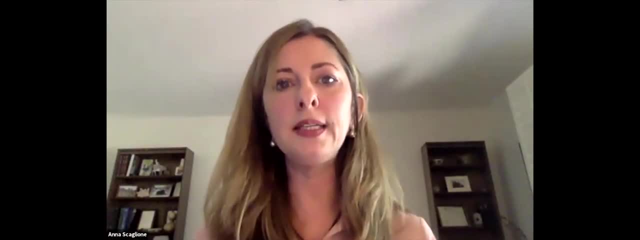 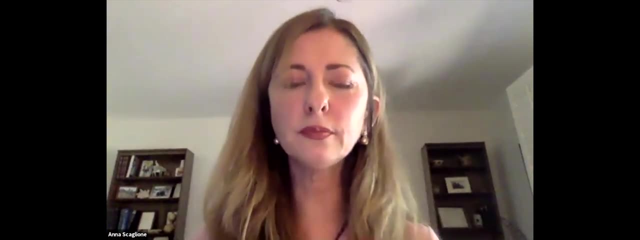 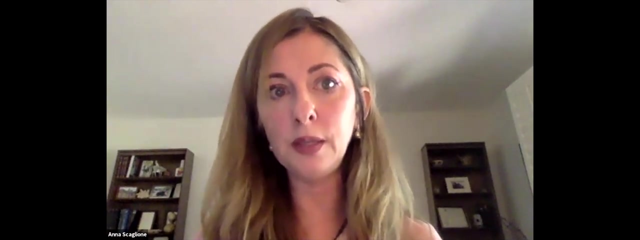 having low dimension. Absolutely, Absolutely. That's really the main point. You know that the result is using the interpolation part. Do there any issues? Are there any issues? Are there any issues with scalability? Well, if you have a very large graph, some of these problems. 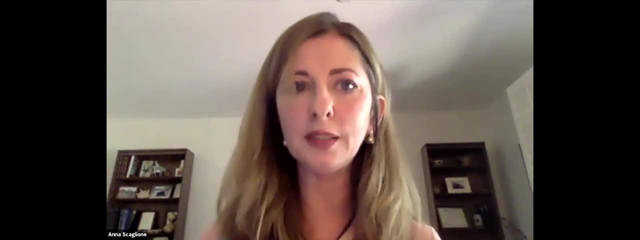 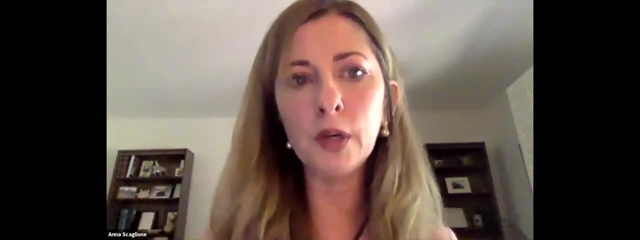 may be daunting, But there is this pretty property that if you decimate the signal, you actually have still a graph signal, And most cases you are not going to have a complete set of measurements for every bus, So you will be forced to do that. 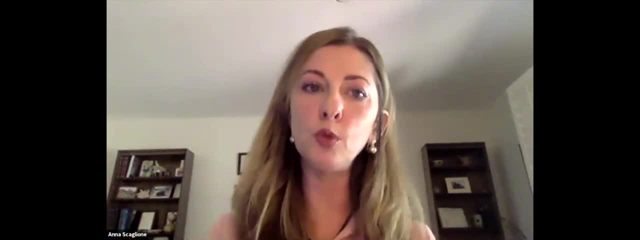 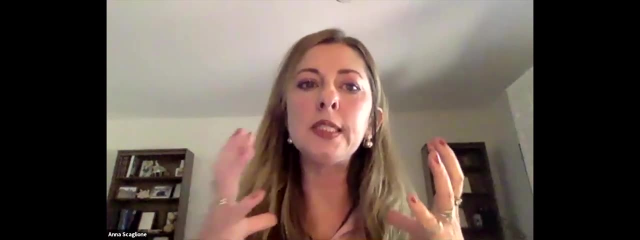 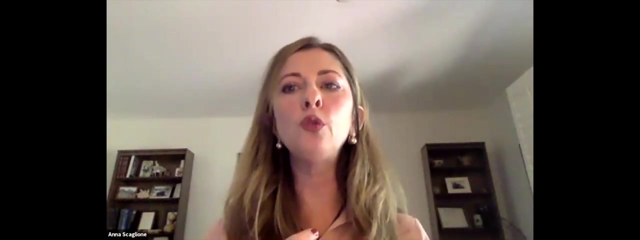 The other interesting divide and conquer approach is by breaking the system in communities. What graph signal processing also shows is very little impact if these communities is quite is loosely connected with another community, So you could essentially consider the impact of other communities as a perturbation. 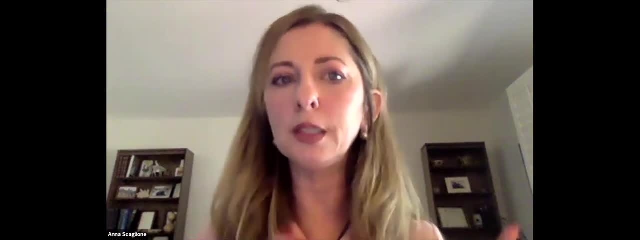 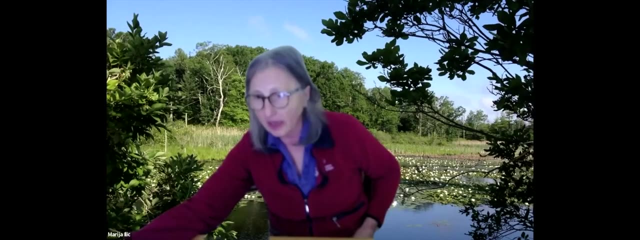 And most of these results could be applied approximately to just a cluster of the grid. So basically, I think the last one is the comment. It says: in low dimensional space- corrupted noise, you may not expect independent projections to eigenvector analysis. 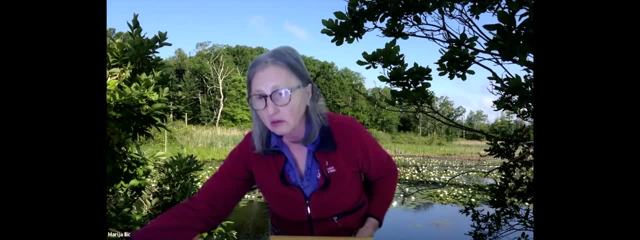 I think you just answered that. You said if the coupling is weak you can stay OK. Any other questions for Anna? OK, so, Anna, I was intrigued throughout the whole talk, But I think you sort of tackled it at the end. 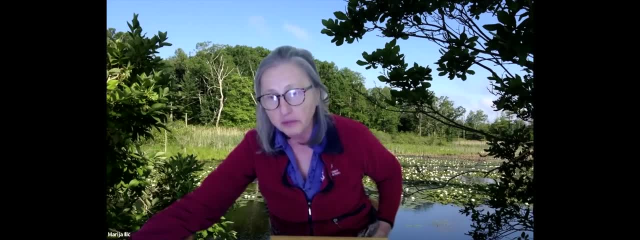 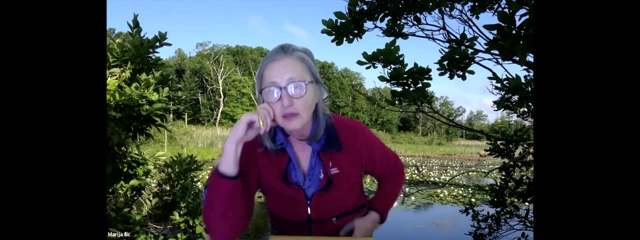 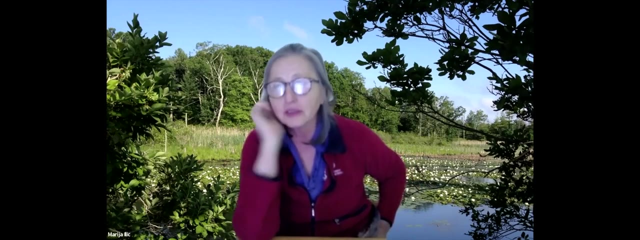 I think what you were talking about is signal processing for data processing, And then you are leaving, And then you are leaving as an open question as future work using a graph theory for physical systems. That was one of the open questions, So I want to ask the question. 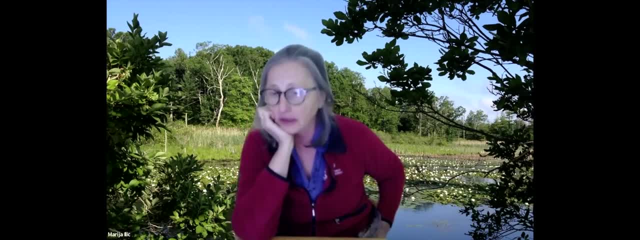 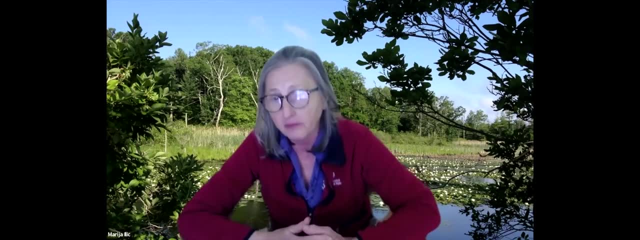 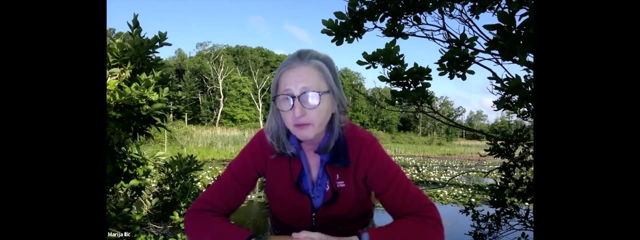 It's really one that we've been struggling with, And I want to point out in particular, the work by late Jan Williams. I'm sure that, Tamer, when we get to discussion, we can return to this question, But when you model physical systems, 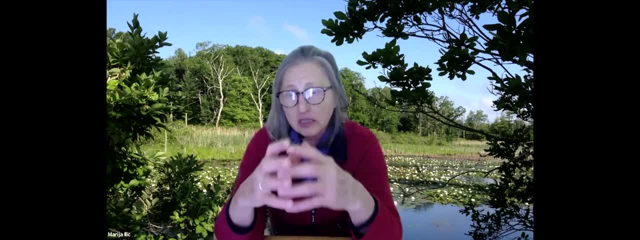 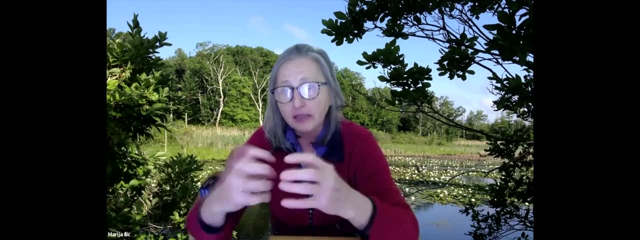 he argues very heavily that the model of the module is not complete. if you just say there is input and output, There are these shared variables that affect each other, They affect the modules, So basically the input-output signal. these are the huge messages. 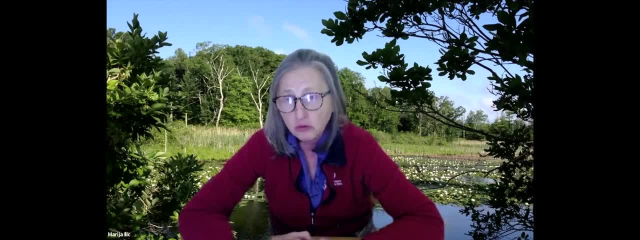 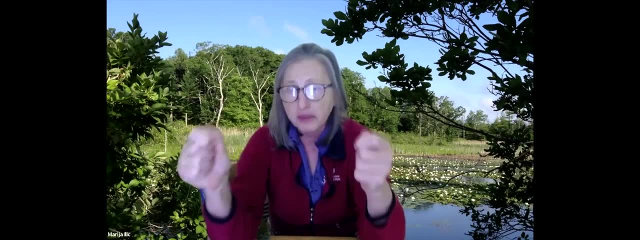 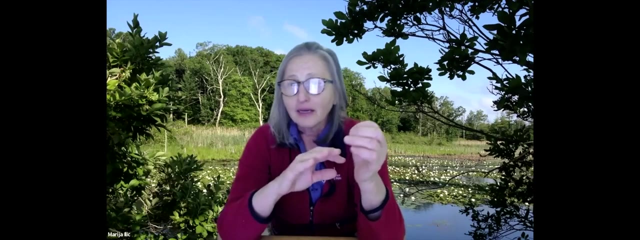 I don't know if you're familiar with Williams' work, But to me it's made me think a lot, And so think about transmission line. Just a very simple example: The way the physical process takes place. you have electromagnetic wave that goes one way. 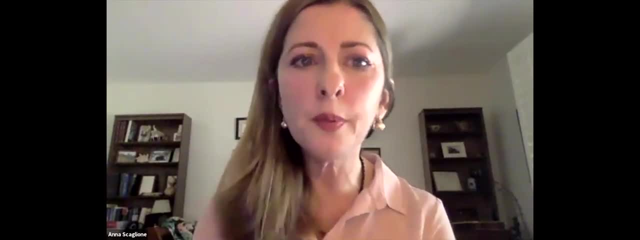 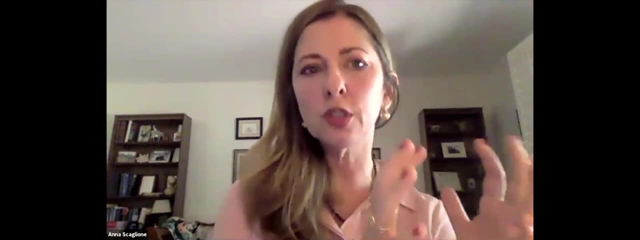 and the other one is reflected, So not saying that you want to come. Can I interrupt you one second? This whole problem was taking the conventional physical equations that are used to analyze grid signals, sorry, to analyze voltage phasors. so, Ohm's law. 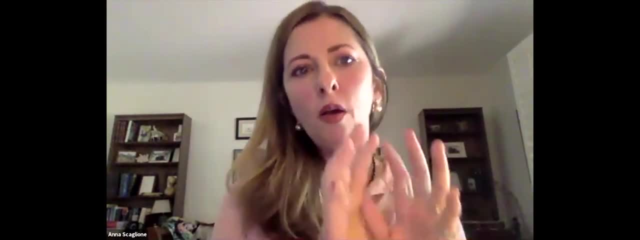 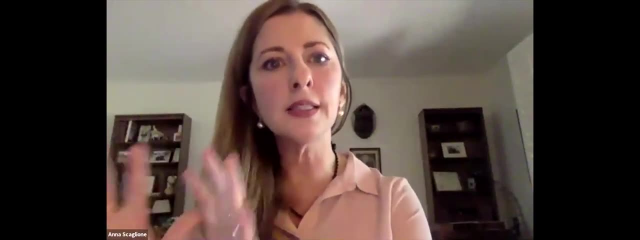 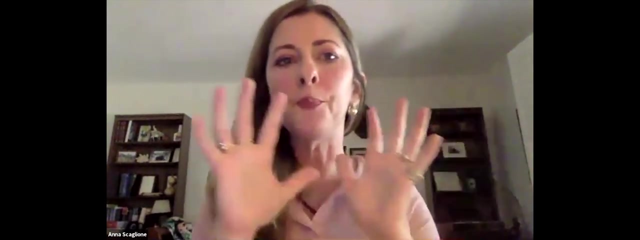 generator, dynamic net or so on. The physics Is there is to say, if you take this physics and look at them under this lens and understand how to connect it to a graph signal processing. So the physics is that the physics for the grid. 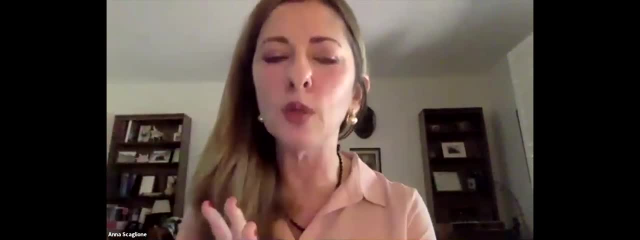 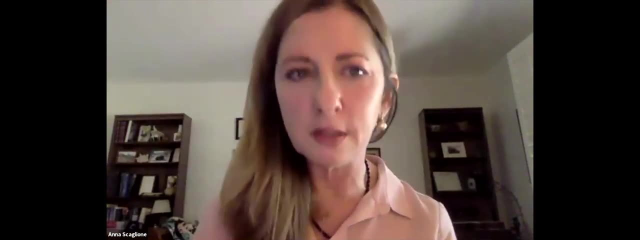 But the idea is to do this mapping Because once you understand what the mapping is, you can just pick and choose tools that have been developed in this field. You don't have to rediscover them in the grid. So let me say, Let me finish my question, and I really 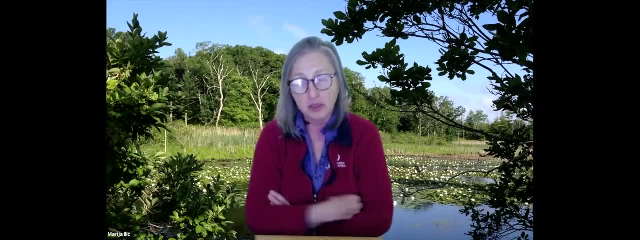 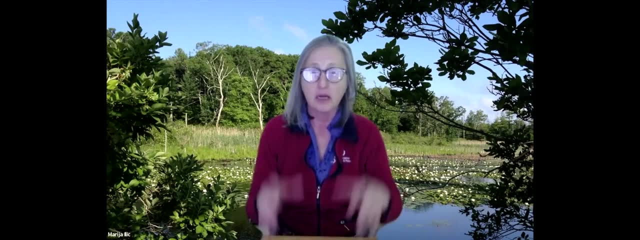 would like to urge the community to think about this, Because I don't understand it fully, but I think it's a very important aspect of what we have in the changing industry. You cannot go module by module and say, doesn't matter what the physics is in. 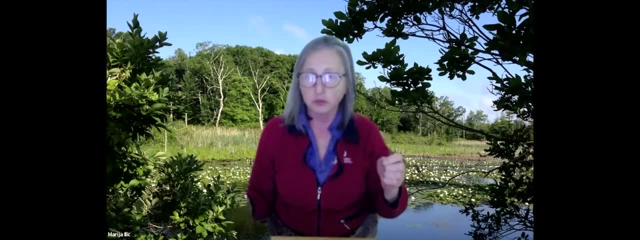 There is directly defined input and output. What signal processing models are based on? Simulink is based on? If you look at the physical thing, there are interactions. There are interactions between the components. So let's leave it at that. Let's we can take it offline. 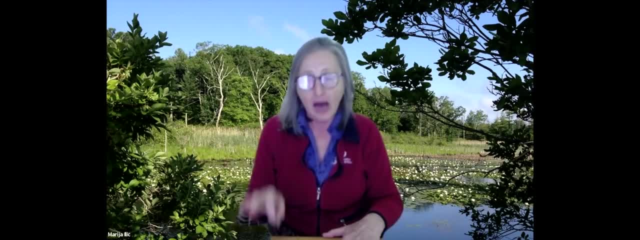 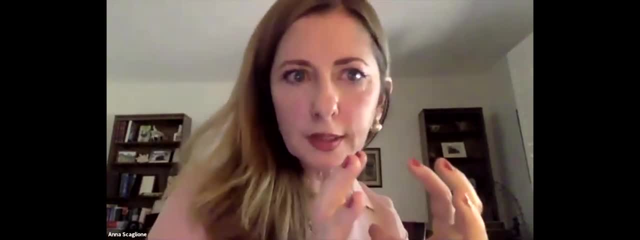 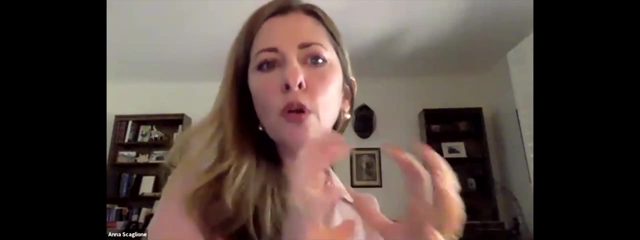 But I think there is a question on the table: How far can you apply that? So the question on the table to me is: you can use this as a feature extraction. The feature should capture all these other underlying processes that are external, So you don't use only the physics.